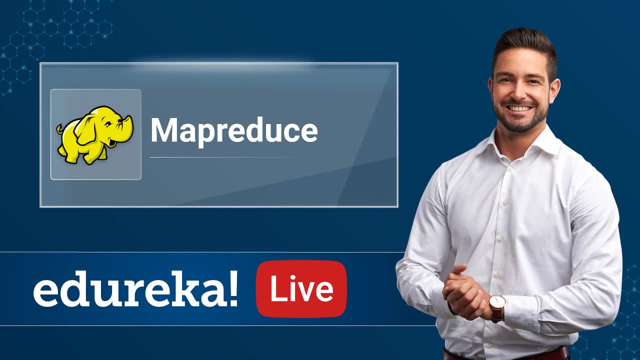 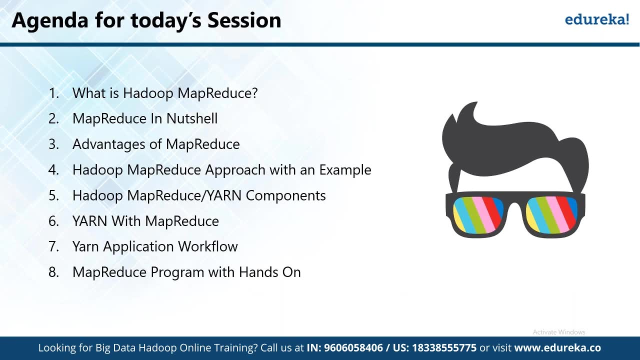 So the main agenda for today's session is: we are going to discuss on what exactly is Hadoop MapReduce. We are going to discuss the logic of MapReduce in a nutshell. Then we are going to discuss the advantages of MapReduce- Hadoop MapReduce approach- with an example. 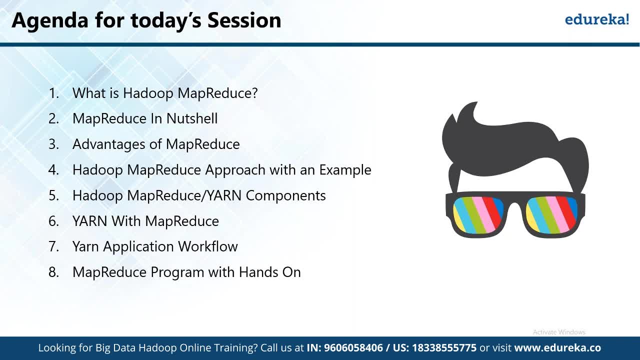 We are going to discuss the advantages, we are going to discuss the map reduce and yard components, yarn with MapReduce, the entire yarn application workflow, and we are going to write a map map reduce program, That means a marker, a mapper program, the user program, one by one. 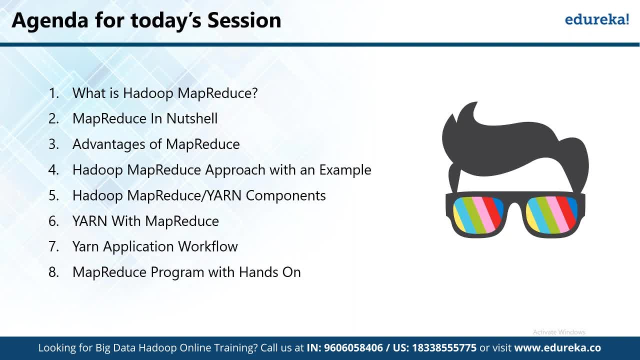 Do we have a complete signing? Okay, how these in different program statements are designed here. So that's the main agenda for this session that we are going to focus on. So, first of all, Hadoop has two components in terms of how to pass. 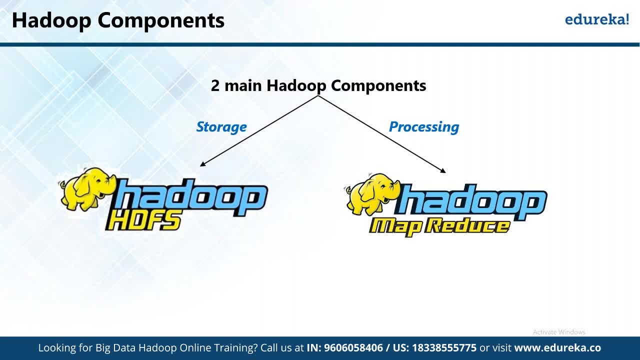 you know, Hadoop is one of the main drivers for big data analysis, for big data engineering and Hadoop. and now, first of all, if you talk about big data itself- and big data can be termed as the class load We can say if we have a requirement of processing, 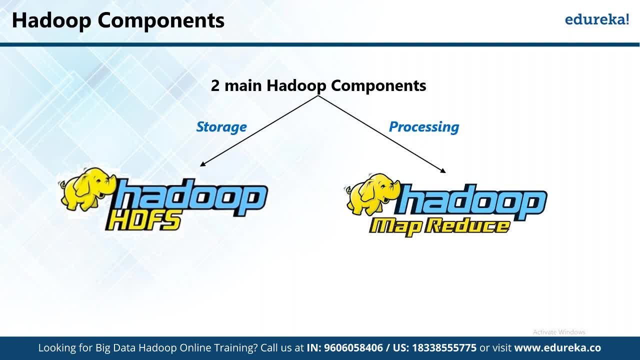 or we can say for fetching petabyte scale of data from multiple sources and that open, we have a complete raw data set available. For example, let's say, when we are trying to provide the analysis on the data stored in the black box for a, for a simple flight correct. 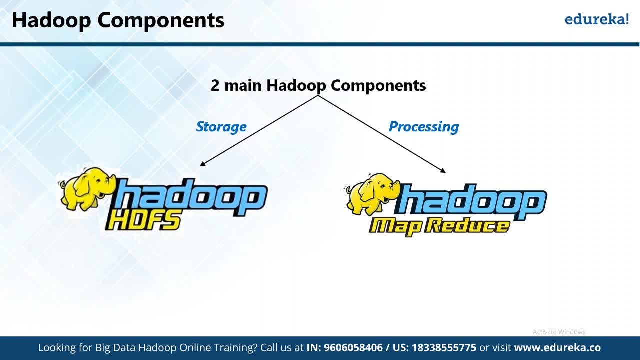 and that black box contains petabyte scale of data, which contains the sensors data, all the all, the cockpit recorder, We can say voice recorders as well. So that is a huge amount of data that needs to be processed and apart from that, we have multi, we have petabyte scale. 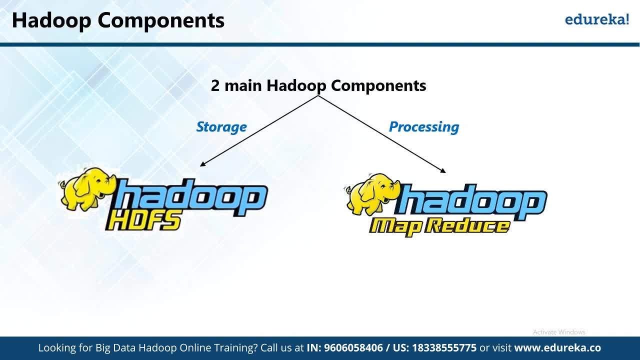 of in-flight data with us, when we have data sets coming in from different sensors, be from the air traffic control as well. So this about this entire piece of data First of all needs to be mined from these sensors and from multiple Hardwares, and they need to be processed first. 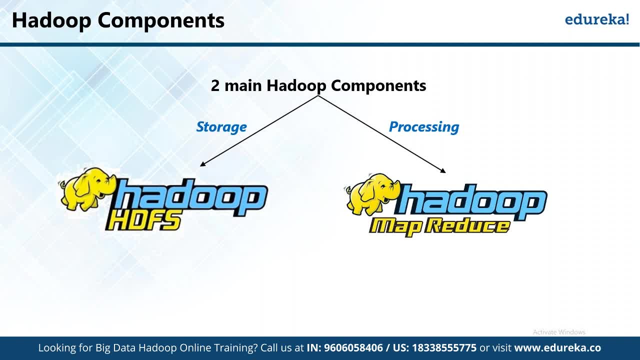 and they need to be stored in different, in multiple locations and in distributed location So then whenever we required to process that data, we can fetch it as quickly as possible. So the main come, the main reason of using beta is to reduce the time which is required. 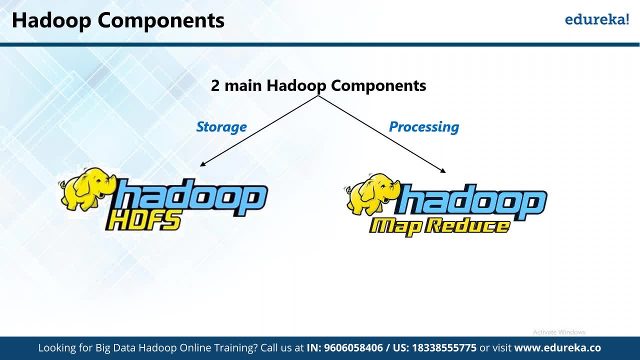 for for the analysis of petabyte scale of data. So that's supposed for, let's say, for processing 1 TB of data using the conventional methods. We need, Let's suppose, five days. then using the Hadoop technology, We can process that 1 TB of data within few hours. 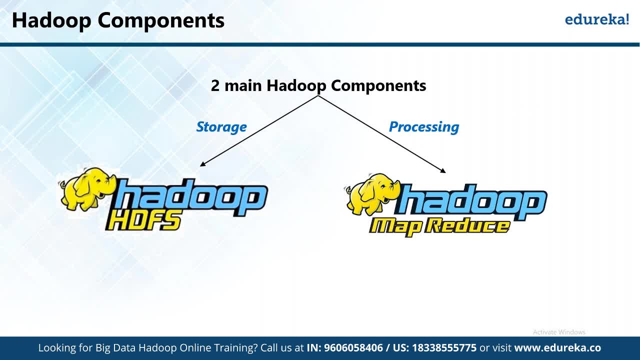 That is a fee- has how fast it makes entire entire data analysis job. And Hadoop? Hadoop is a big data framework with the has been designed and deployed by Apache Foundation, So basically it is an open source software utility that works in the network of computers in parallel. 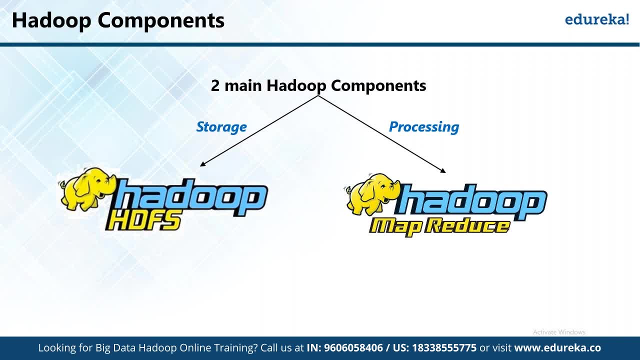 to find solutions to big data and process it using the MapReduce algorithm. All right, and my and Hadoop has two main structures. We have Hadoop HDFS as an Hadoop distributed file system and then we have Hadoop MapReduce. So HDFS refers to storage of the entire data set. 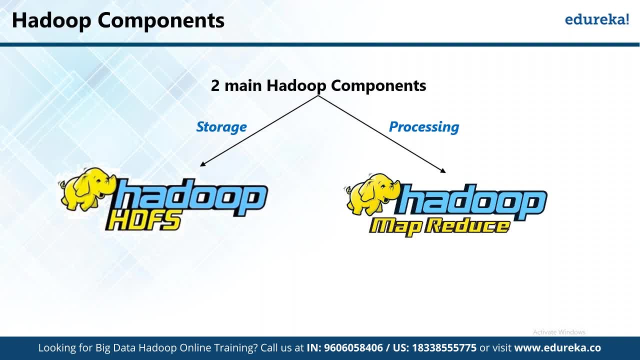 into parallel distribution, For example, if we are provide, if we have a requirement, or storing, let's say, 10 DB of data. So either we can choose to store the entire 10 DB in a single system, They can choose to store the data in a single system. 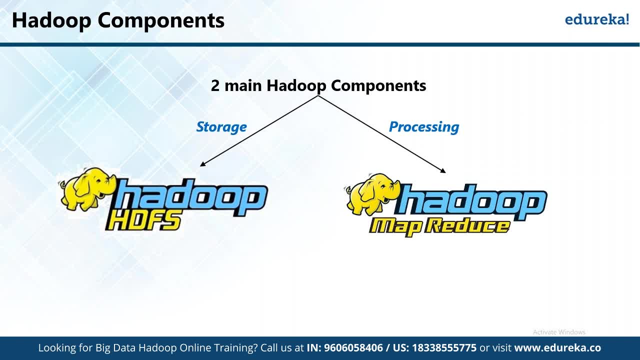 in a single node or we can store the data in multiple nodes and that to parallel so that when we have a requirement of processing that button, TV of data, So as I leave a requirement of processing only 1 TB of out of that in TV- 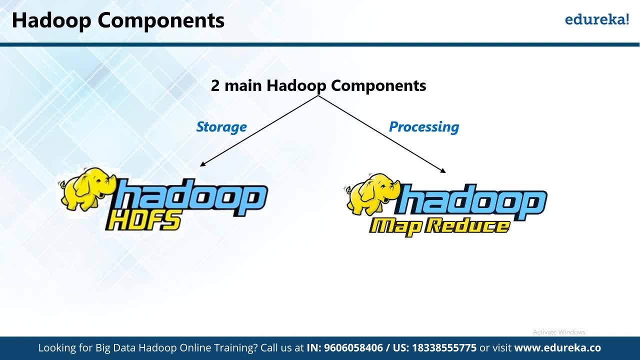 then we can use, then we can refer to that particular node, that particular size, in which we have 1 DB of data stored, so that we don't have to worry about setting up the entire, We don't have to study, worry about setting up the entire. 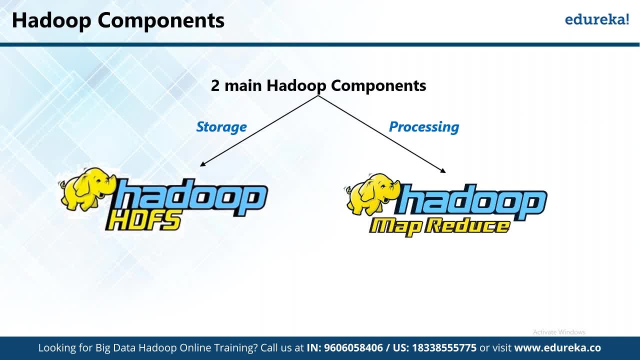 or gets it looking for the entire 10 DB of data for just for putting that piece of information, of information in which we are interested, Right. and then we have MapReduce of Bab reduces, basically used for parallel processing If you want to process the data parallelly. 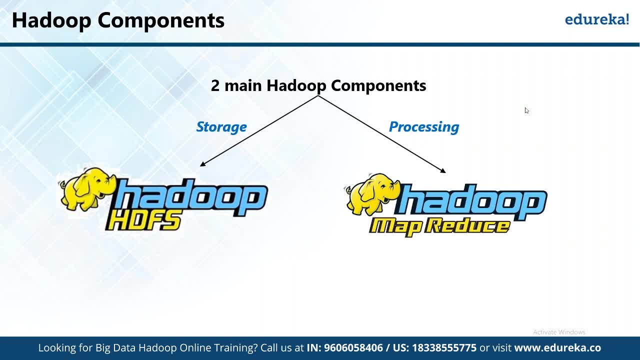 we want to get the inside out of it parallelly without spending much more time. Then we can distribute the entire world. For example we have- we are using one system prepared to process 10 TB of data. So instead of using a single system to process 10 TB of data, 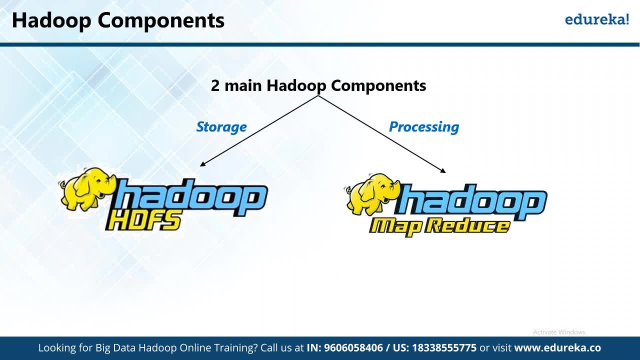 we can divine that we can divide first of all 10 DB into 1 DB each and then we can assign each 1 DB to a separate processor so that the entire process, the entire time required for processing, can be lowered down. If you all remember back in a school days, 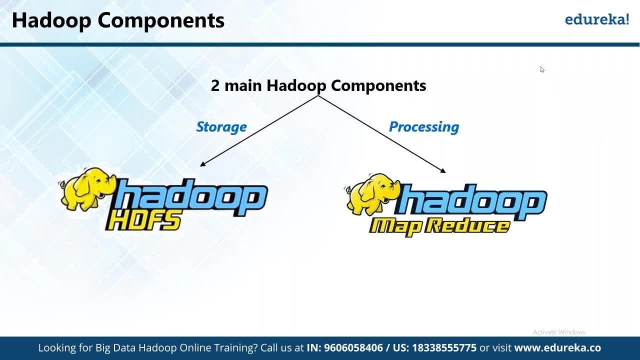 we had multiple problem statements. that was: if a worker X takes 10 days in order to complete Complete a bridge, then how much? then how many days will 10 workers need to in order to complete the same bridge, correct? So the same process again. we are what we are doing. 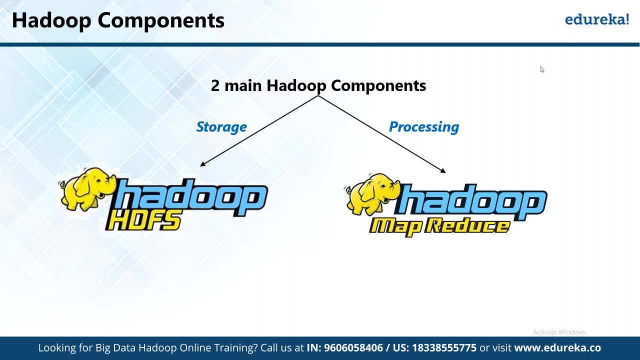 We are distributing the entire work into multiple workers. Same process is followed by SGFS as well. So instead of going for singles, we can see a single node and single processor. We divide the entire work into smaller work and then we hire multiple workforce, or in this case: 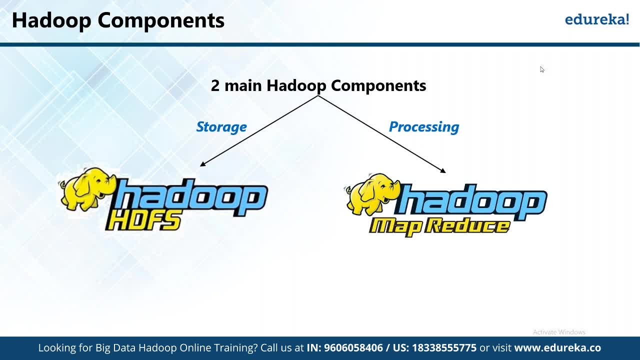 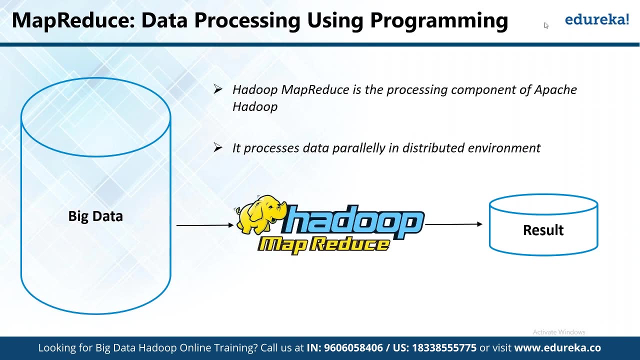 We hire multiple Nodes of against a multiple processors for processing that large piece of data for us That we achieved by using the components of Hadoop And Hadoop MapReduce. as we discuss again, it is simply processing the component of Hadoop and it provides the parallel processing. 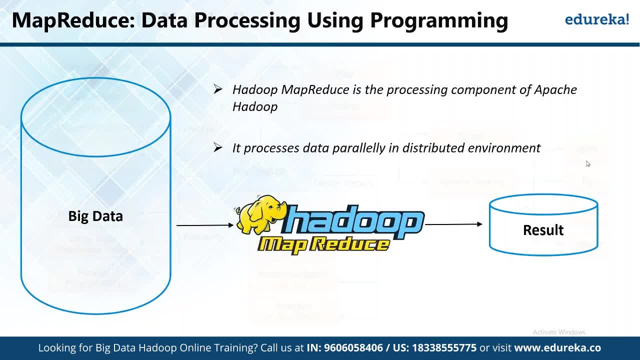 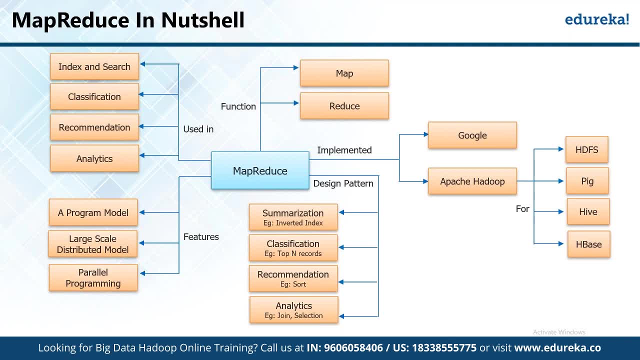 of data in a distributed environment And MapReduce in a nutshell. So first of all, the MapReduce is again, if we have to analyze MapReduce in simple lemon dust, for example, if we have to understand the entire components of big data and with simple example, 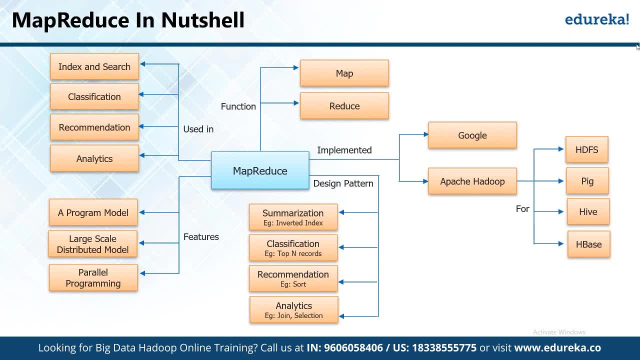 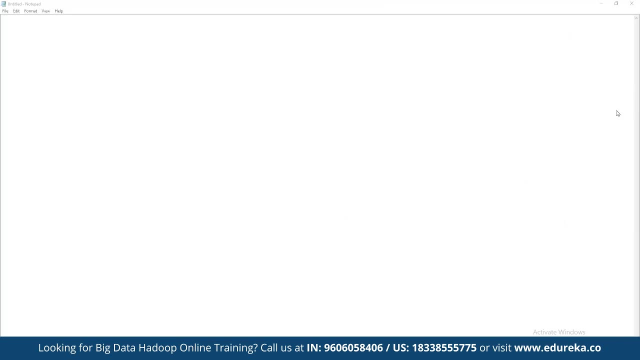 let's do that Before we go into the technicalities. let's start a simple example here, So that we can focus on these technicalities in a much better way. Now let's move on to our Picasso models as our hands-on. 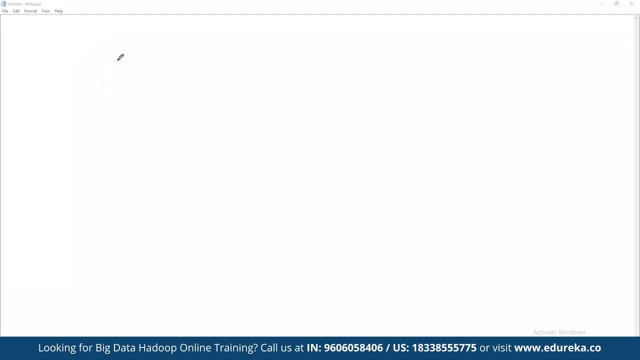 Now let's understand. the main idea behind big data is EFS and MapReduce. Let's say we have a requirement of processing A thousand page book. Now, This is a thousand page book, and in these thousand page book, in this thousand page book, 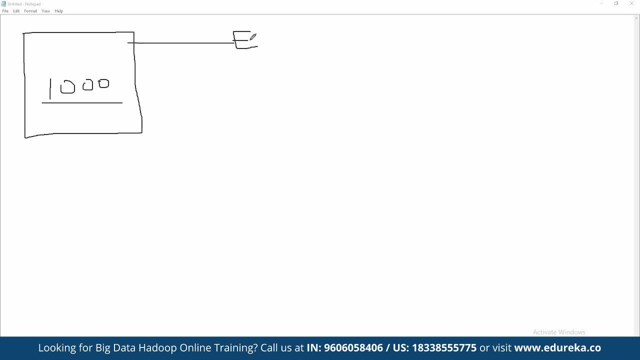 We have to analyze how many times the word edureka, for example, how many times word edureka appears in this thousand page book. This is our problem statement and for getting this right We have four students with us: one, two, three and four. 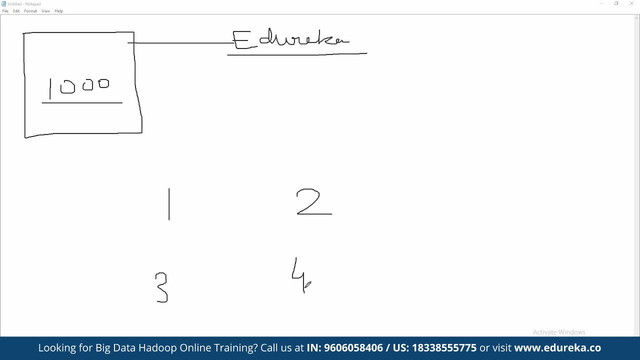 We have had four students with us and to make things simpler, What we have done, We have given, we have made four copies, or the same thousand page book. We had the first copy to student one, second copy to student to third copy to student three. 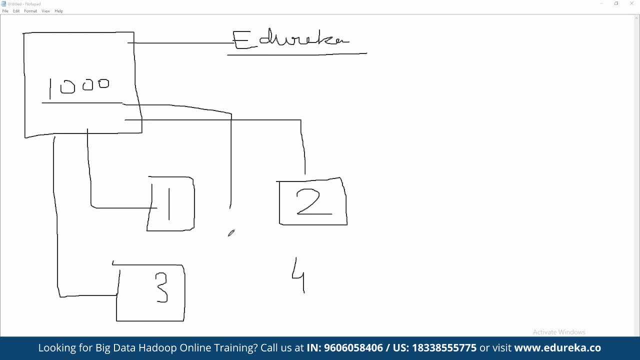 and so on. the fourth copy given to the string for that piece. They all have the copy of the same book, that is thousand pages, and now each and every student- Suppose each and every student here, the student took four hours in order to read the thousand pages. 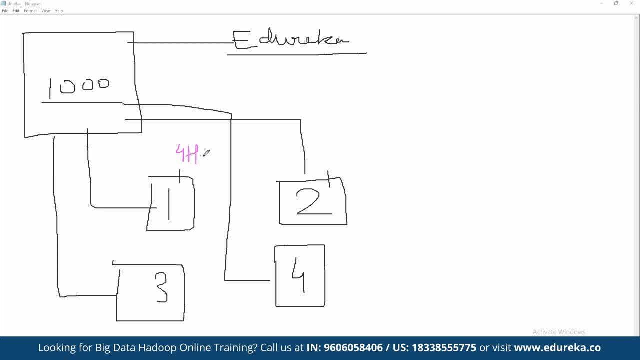 to agent a student. It took four hours each in order to read the thousand pages. So you are so serious. one thought: four hours is 224 hours, use A: 324 hours and so on. so each and every users. they took four hours each in order to read the G through. 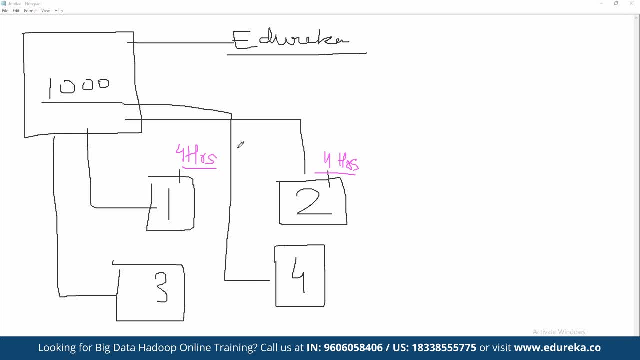 going us to go through these thousand pages, all 6,000 pages, and after four hours of analysis they came with the result. That is, for example, the first user, the first student came the result, that word Erica, appears 42 times. same way user to give the result. 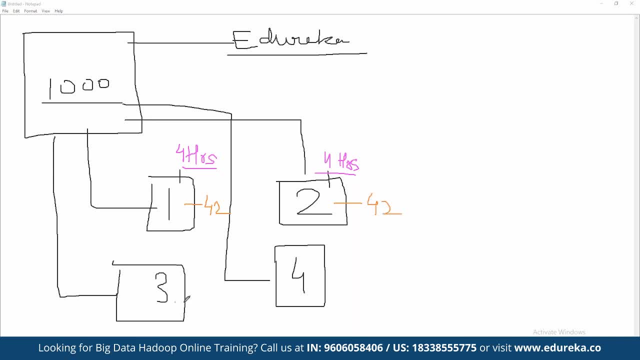 as word and Erica appears for you to follow two times user 3k. the result out of four hours, 42 times and user 4k- there is a suppose as 41, but collectively what we had done, We have simply map the entire results together. 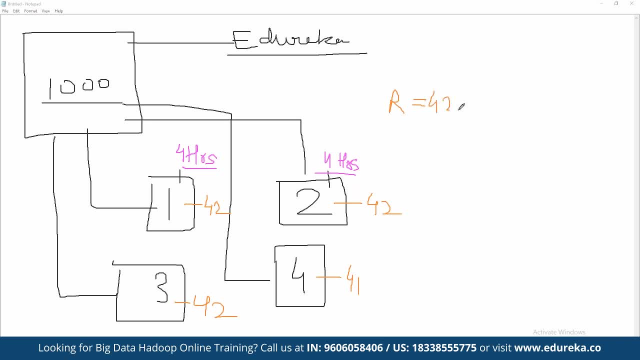 So result is 42, and the time required for this analysis was 4 hours. 4 hours plus couple of minutes in order to compile the entire results together as well. Correct, So for processing thousand-page book, be here. We took almost four hours into prefer. 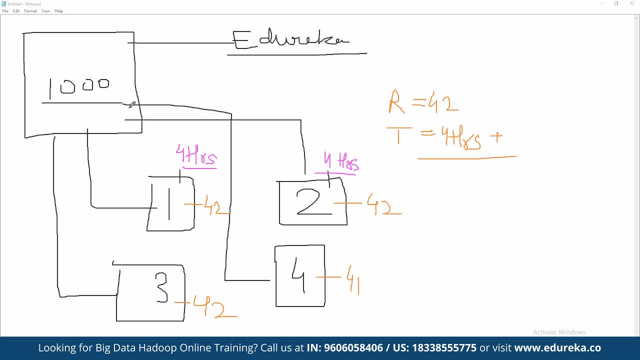 into. we can say, primary analysis for the same book. right now The same thing can be done in a different way as well. So how we can do that. Let's understand that part. Let's say we have the same use case We have. 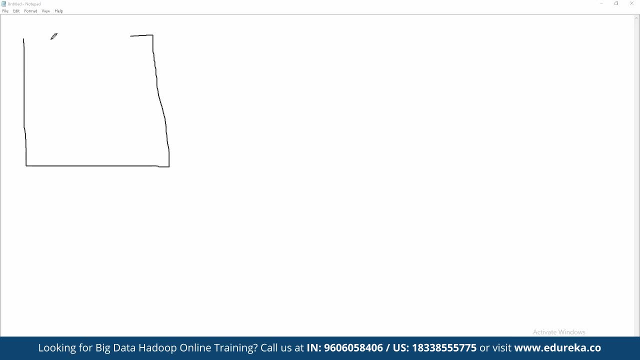 the same use case as a thousand-page book. We have same use case as a thousand-page book And now, instead of giving the entire thousand pages was the same way. We have four students, So a certain one, two, three and four. now same prone statement. 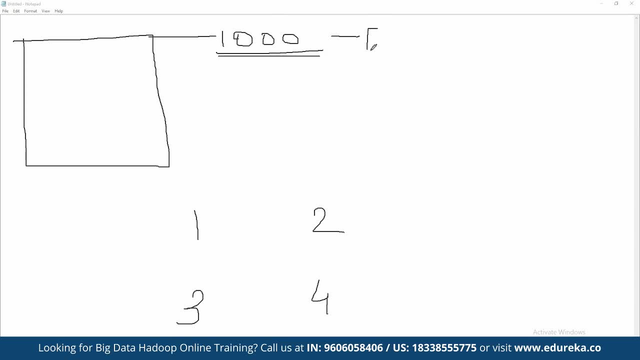 We had to find out from these thousand pages How many times the word edureka appears in these thousand pages. right now, here, in this scenario, instead of handing over the entire thousand pages to each and every student individually, what we do? we take the help of HDFS, as in distributed file system. 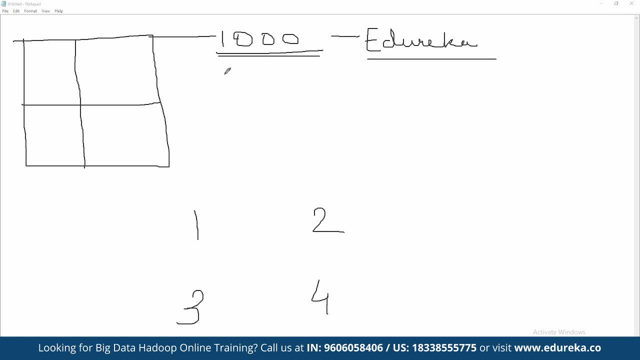 or we can say, distribution of the entire data set. So instead of handling over the entire thousand page, what we have done? we created multiple sections. That be the first section. the first group contains 250 pages, The first 250. the second group contains the another 250 pages. 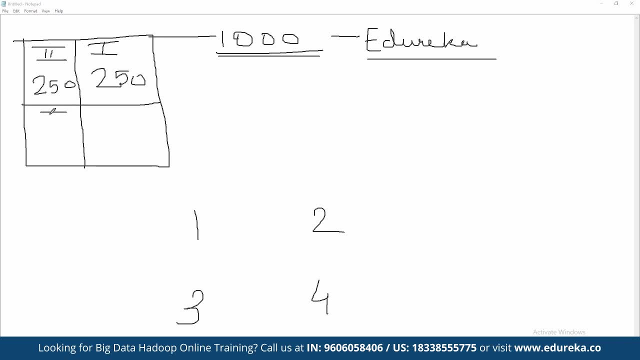 That means after the first module, The third group contains the next 250 pages and same before the fourth bottle. fourth model also contains the next 250 pages. So now the entire thousand big page book has been divided separately to four different components. having the old set, 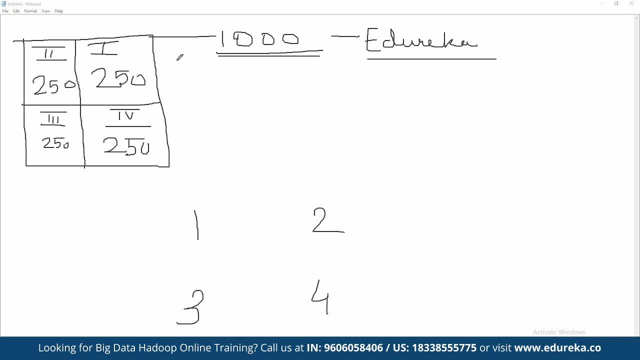 of 250 pages right now. each and every set is now given to an individual and I can say users. so user one, or can say student one, got the first set, student to got the second step, the second set, student tree- got the third set, as in third set here, and student for got the fourth set. 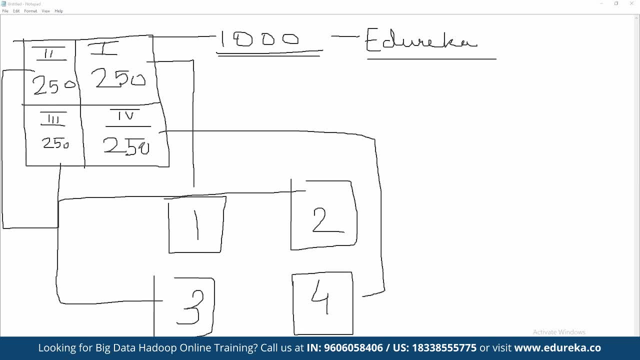 So now each and every student had they have to analyze only 250 pages, not more than that. So now for going to 250 pages. suppose user not each and every student, It did took almost one hour each. They took almost one hour each in order to go. 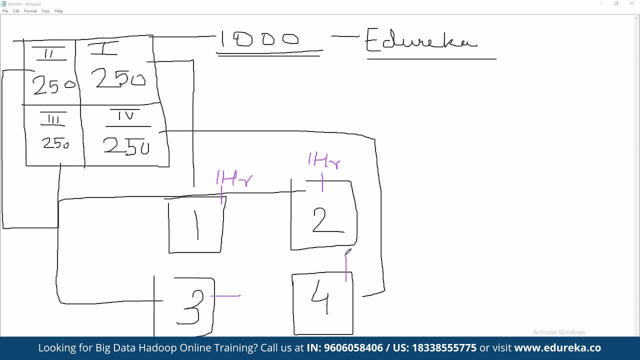 through the entire set of 250 pages right now, after one hour of analysis. now, user one gave the result: Okay, it appears 12 times. user to gave the result: Okay, it appears 10 times. user 3 also gave the result as 10 times and user 4 also gave the results. 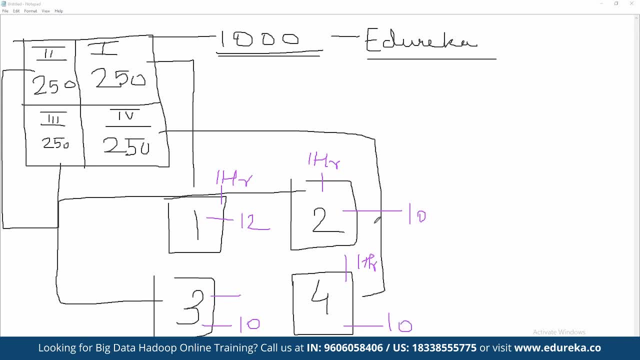 at 10 times in their respective set of pages. So now, what we can do using the map reducer. what we have done? We can simply map the results from each and every instance together, So we can say that 12 plus 10 plus 10 plus 10 is going. 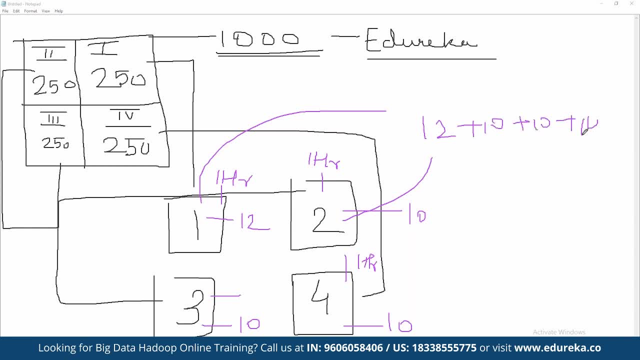 to give us a result as 42, as 42 that means in that result. Here is what: the result here is 42 and for the entire analysis of this number we have, we have spent only how much? one hour plus few minutes, all because of the parallel distribution. 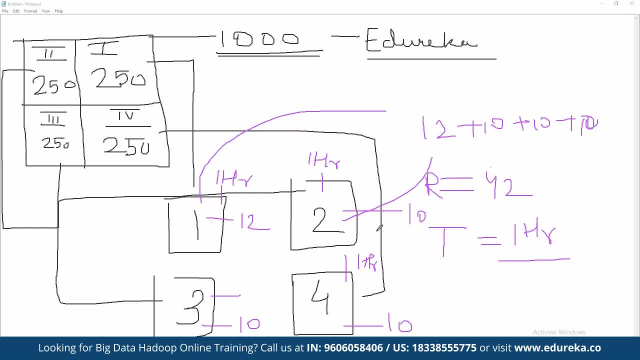 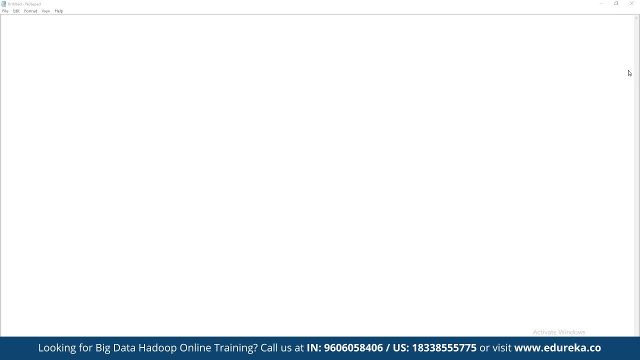 and going for going for Map reduce framework as well. So that's how the entire concept, for that's why we use big data. So simply reduce with a single goal of reducing the time of the entire analysis, because without big data also the analysis can be done. 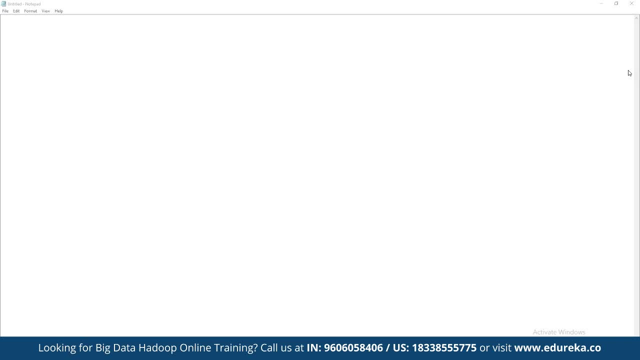 It was being done, But again it would took forever to process large scales of data sheets or reassets. All right, so now these are the different components for map, for map reduce. So first of all I give MapReduce are used is used in indexing. 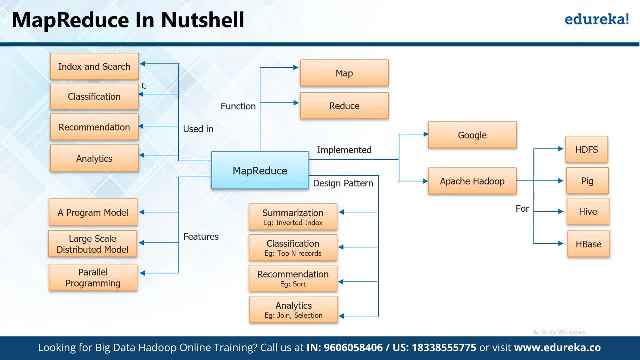 and searching for classification, recommendation, analytics. It has the features such as a program model, large-scale distributed model, parallel programming and has in terms of design pattern. It uses the civilization, as in the inverted index. It uses a classification, recommendation and analytics and down to the function. 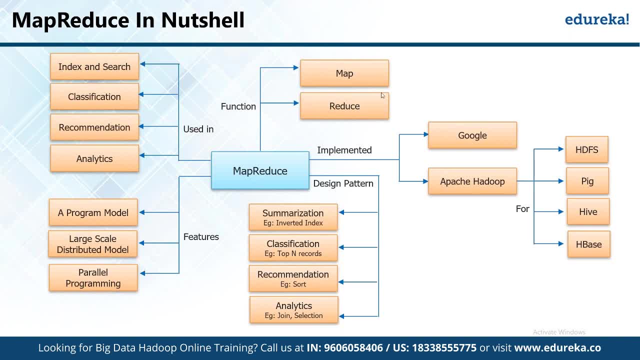 It has two functions: one for mapping and one for reducer. So we are going to still look at both mapper and reducer function, because when we are adding the MapReduce code we have to write separate code for mapper and separate code for reducer. that is we are going to look at. 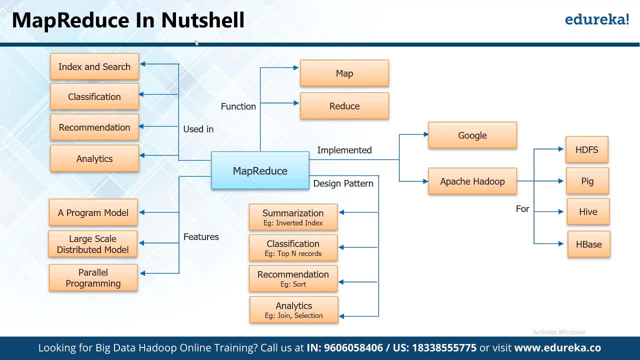 Now, in terms of the, in terms where it is implemented or give it is going to, it is well implemented and Google and the entire Apache Hadoop and Apache Hadoop- This is used for HDFS, for peg I H base. So now, what exactly are these different components? 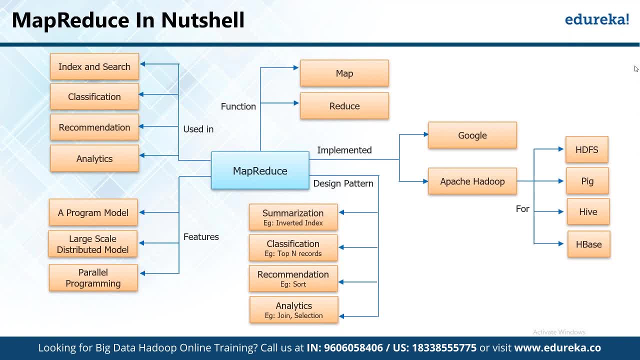 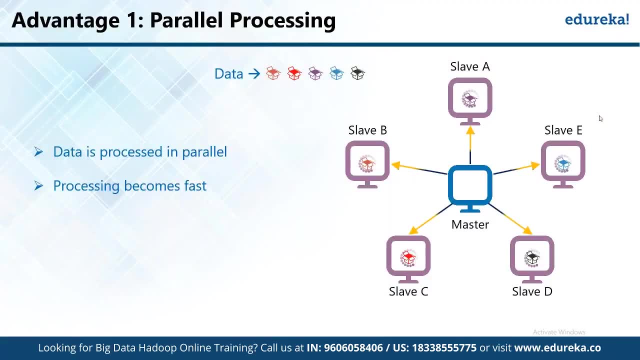 in how to park a lecture. We are going to discuss this part Step-by-step as you move further. now the two biggest advantages of MapReduce: So data is processed and parallel. that we have already seen when we have discussed the use case for our book program. 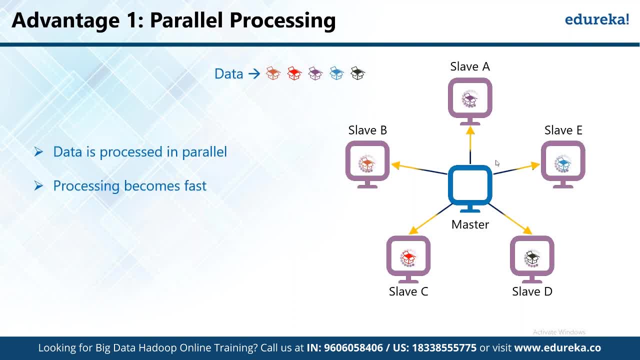 correct and that processing becomes faster because, instead of using just a single node, we are using multiple nodes to provide the processing, and that, too, in the same time. and again, we are not processing the same data, but we are divided. We have divided the entire. 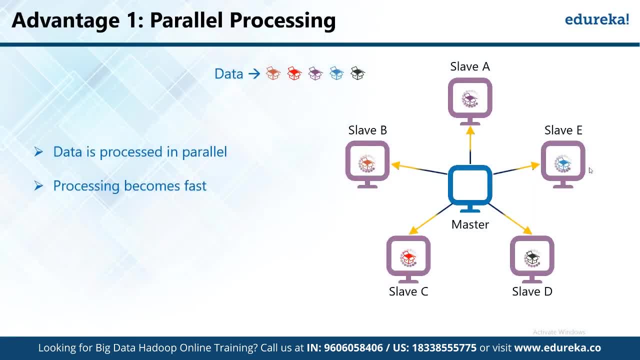 Data into smaller components, and then each and every data packet is being handled by a different slaves. Now here we have a master in slave architecture, So master will decide. for example, we have 10 DB of data, Then it will decide in how many nodes isn't this entire data? 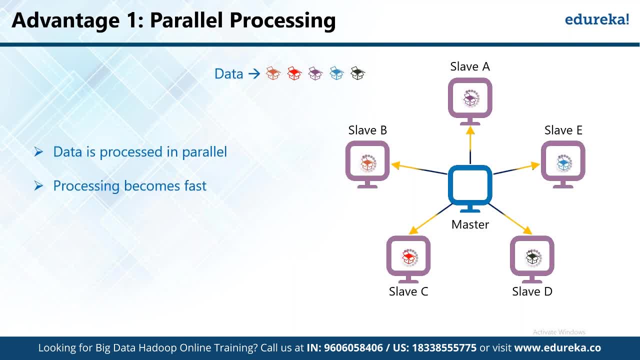 has restored and how exactly they have to be stored. We have to define. we have to define each and every component here, Okay, and then here we define again. for example, we have 10 DB of data. We can create five nodes. 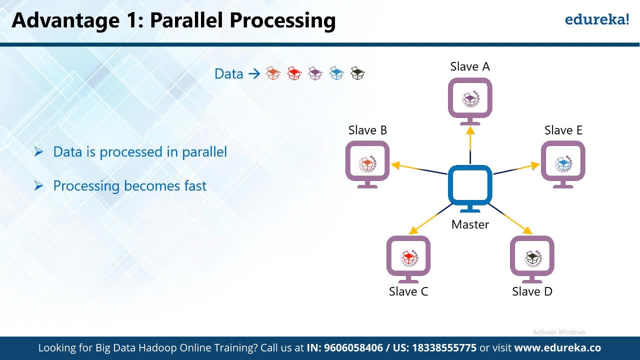 Then we can create an. this is going to create five nodes and then the entire node is going to have different. we can say 1, 1 DB attached each for 5 TV of node and then we are going to process the entire data set parallelly. 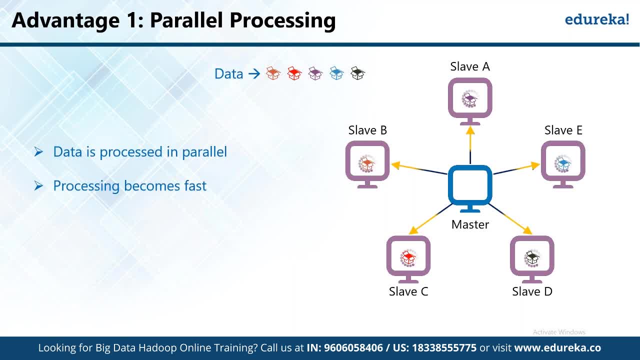 so that in initially, if it takes, let's say, 20 hours, 50 hours to provide the same analysis, Now it can be reduced to forgets it more than five times, because the same processing is now being turned by individual instances, and that too, parallelly. 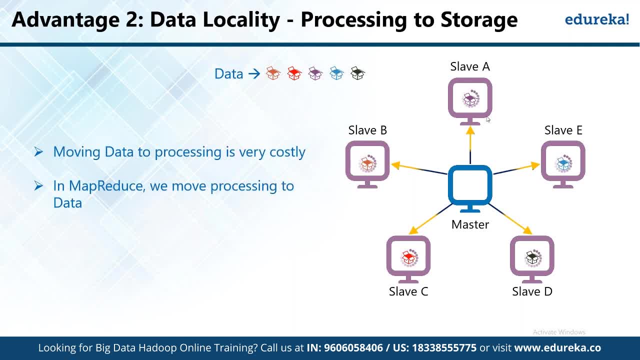 And moving data again, because moving data to processing is very costly. in MapReduce We move processing to data because instead of moving data data to the processing, We are simply moving the data. We are moving the processing to the given data set. That's what exactly. we make sure that in that course. 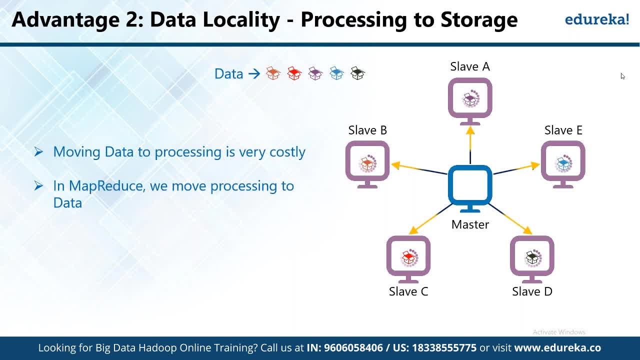 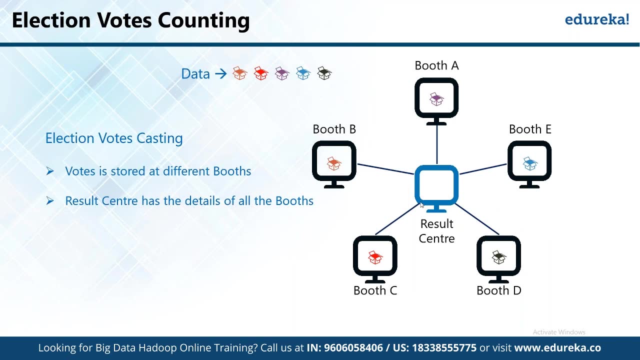 for MapReduce, for this parallel processing is not also going much higher than what we have, What we are client has planned And the traditional versus MapReduce way. the election votes counting now. boards is stored in different boots and result Center has all the details of all the boots available. 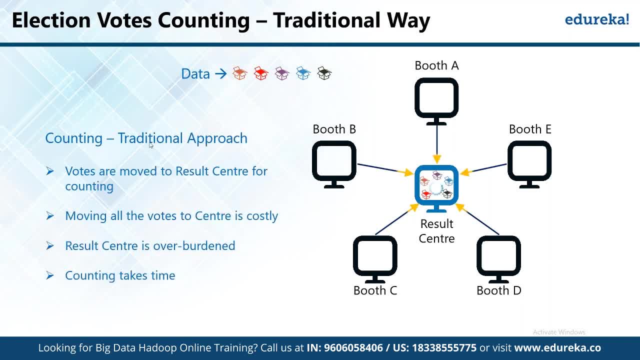 for different boots here and then it can start up counting. in traditional approach The votes are moved from result to data Center for counting and moving all the votes to Center is costly, because suppose if we have 50 DB of data stored in each and every booth and now if you are looking to move 50 DB, 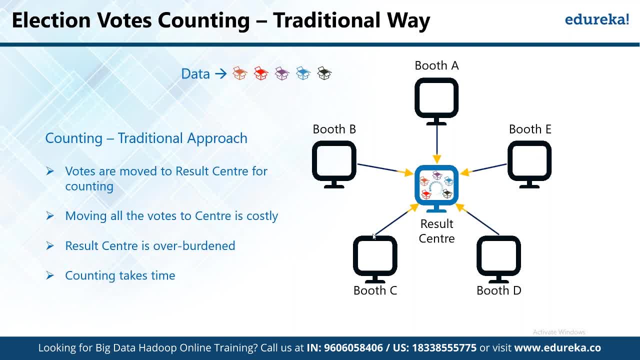 all into a centralized location, and moving that 50 DB of data is also going to be costier. plus, when the entire data set is available in centralized location, Obviously the result Center is going to be overburdened, So this is going to create a situation of bottleneck. 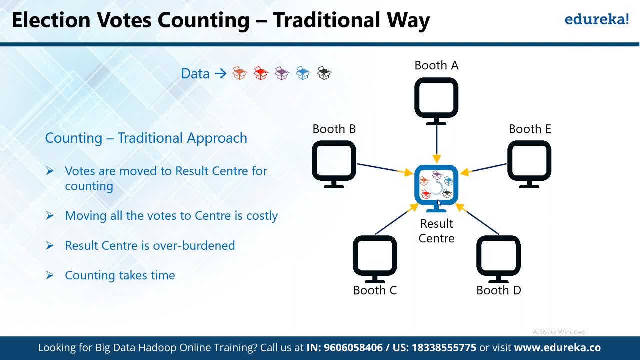 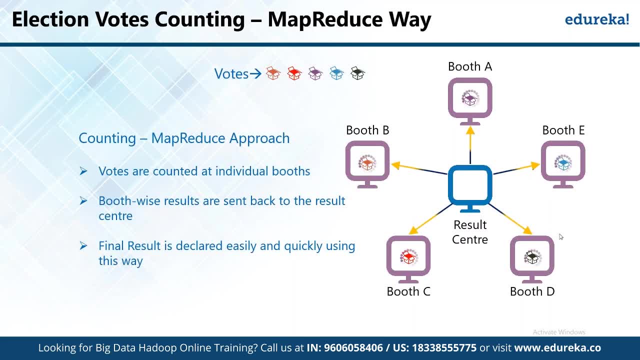 and that's why, if the entire processing is to be done by single data Center, obviously it is going to take time. So, instead of doing that what we do, we allow different data Centers to start processing their own piece of data individually so that, once they are done, was I'm a booth. 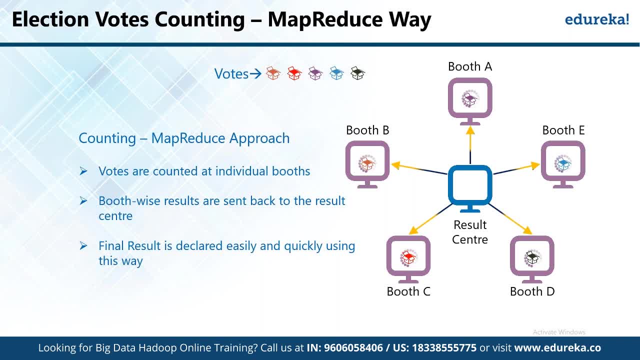 We is done calculating. Now would be calculated Okay for for candidate a it they were supposed 100,000 votes and for Canada be they were 20,000 volts. then you can send the result back to the center. against a result Center, all the master nodes same way. 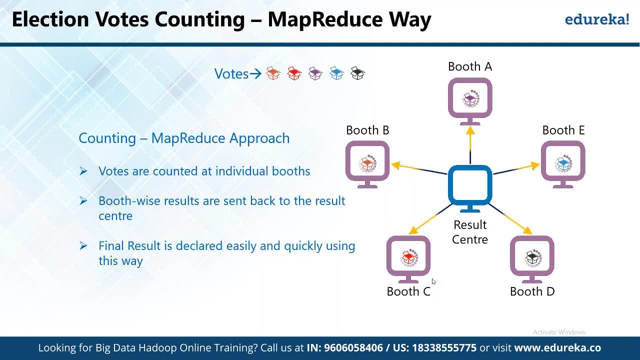 for each and every reason, each and every data Center results can be. the entire processing can be done here only, and now the results can be sent back to the center so that now it can simply club all the results together and then it can showcase the end results. 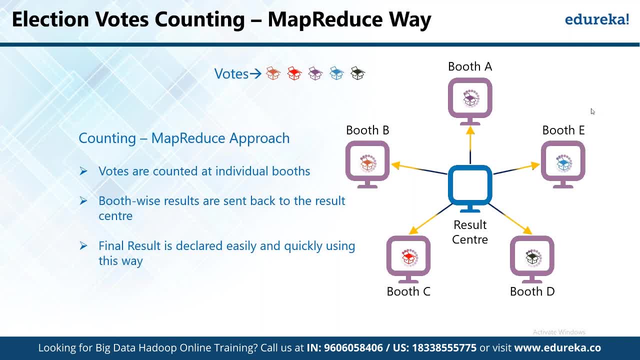 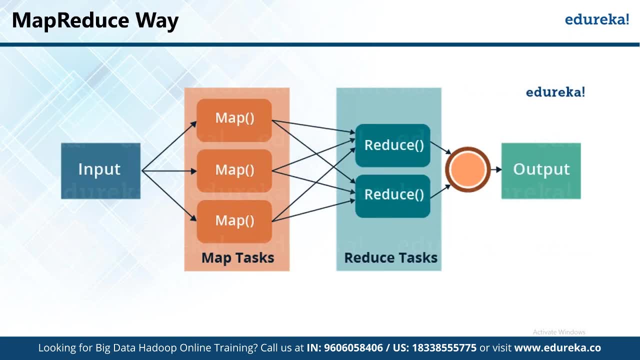 I can't agree to simply reduce the complexities because at the time required for completing the given job, All right. Now the map reduce again. first of all, in MapReduce We give the entire input. So here we have redefined it: multiple data pointers here. 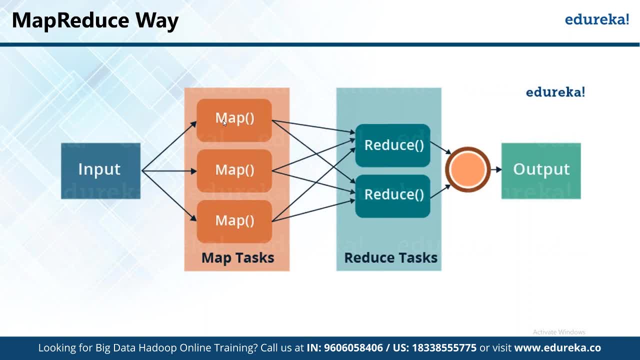 where we have to work on and just know these and then these pattern. they have to work on the data ingestion techniques And then now, for example, of the multiple towers that needs to be mapped here, For example, like we discussed, we have multiple pages that needs to be processed. 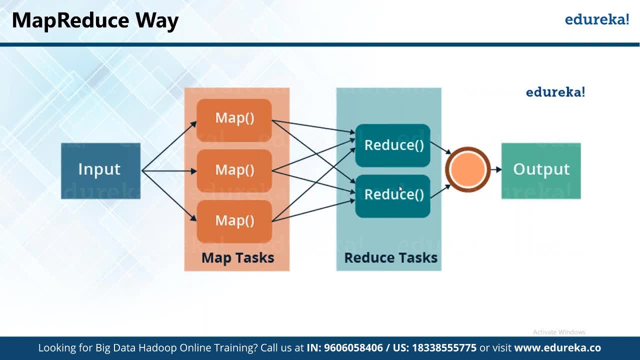 So whatever has been output of the processing, They are being sent to the reducers and then they reduce it. output is single output and then that's how it's being presented to. different individual can say as a final result here, as a part of my party, 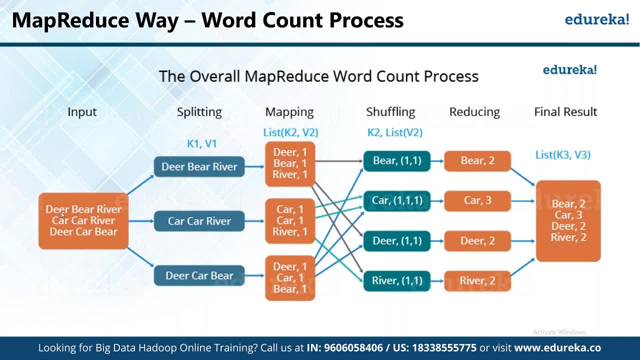 Now let's say, here we install simple use case. We have a simple tag of dear beer River car, Our River video copier. now we want, or we can segregate these and tap this entire free piece of line in separate, one line each, like we have here. 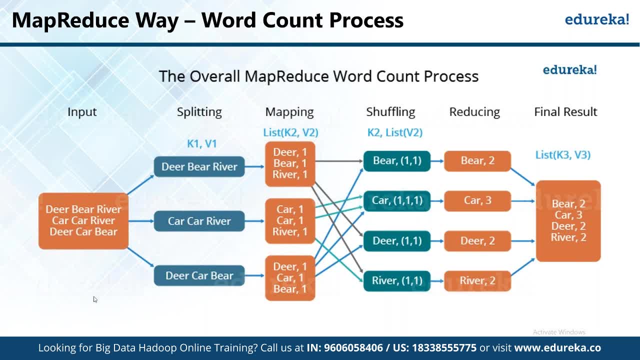 This printout process is called a spitting, When we are defining the entire large regressor into smaller regressor. and we had your beer car River. Now what we have done? we have three separate lines. Now we can again segregate, we can again by forget each. 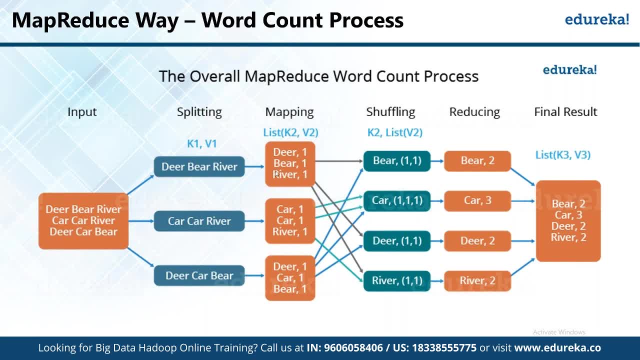 and every of the lines into individual words. like we have dear beer River, We had your bear and River, car car River and your car bear. So we have. we have other components available, available. Then we can define the key. key as in the exact word. 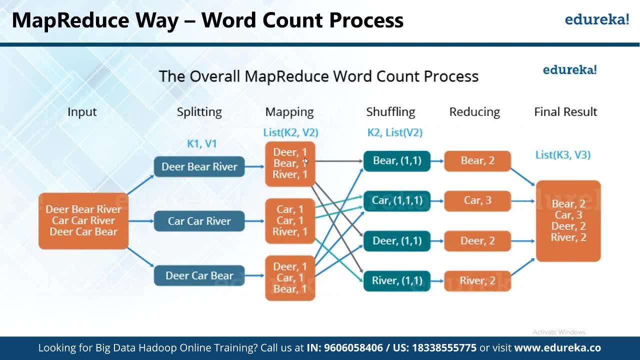 and the value. that means how many times these words are present so we can see: dear is present one time that we have beer, and then we have beer and then we have River. so same big car car, River, dear car bear. Now we can shuffle it. that means I when we say shuffling. 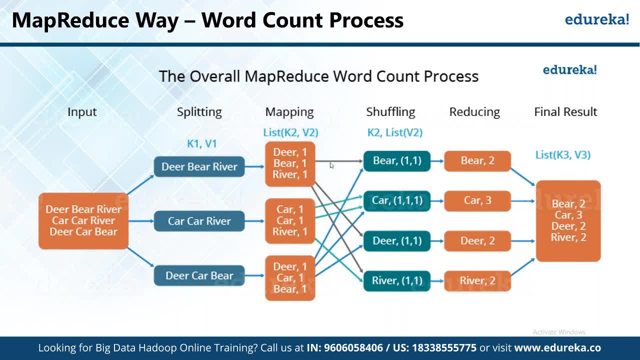 that means now we can segregate these words individually. That means here we can have a separate word for bear, car deal and River. so bear we can pinpoint, suppose. from the first list the word bear appears one time, So you have, we have one. in the second list bear is not present. 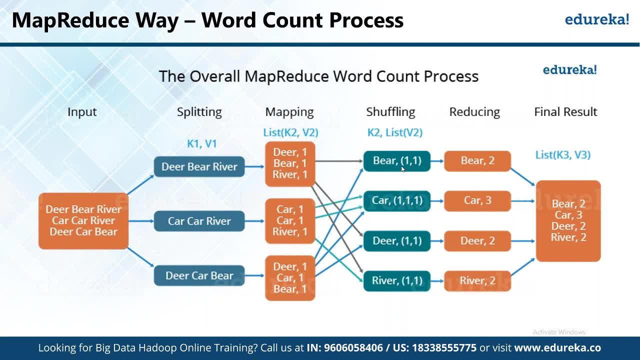 That's all. but in a third list We have bear at present one time. So we have now beer one. one. one. same way for car. in the first list We don't have a car. in second list We have car available two times. 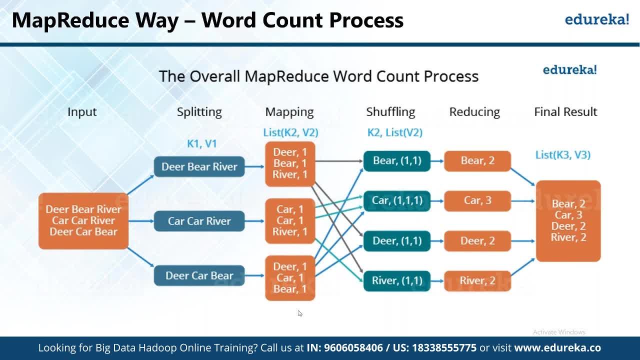 So we have car 1 and 1, and see me in the car. We have one. We have got available one more time in the third list. So we have, we have Carl. one was one more time. same way for dear, for dear we had in the first list. 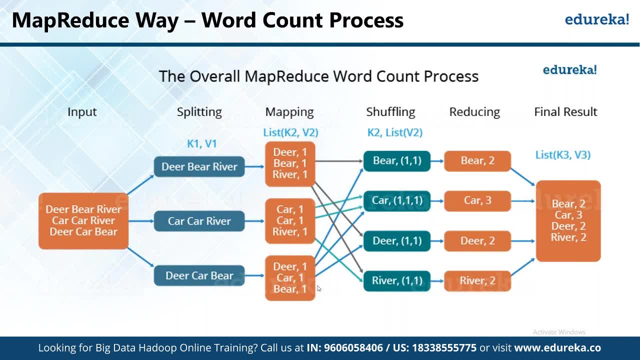 We have dear one time and second is we don't have dear and in third is we have one. Same way for River. We have one time River place in the first listing and the second list as well, but not the third list. So that means here we have simply shuffle the entire words. 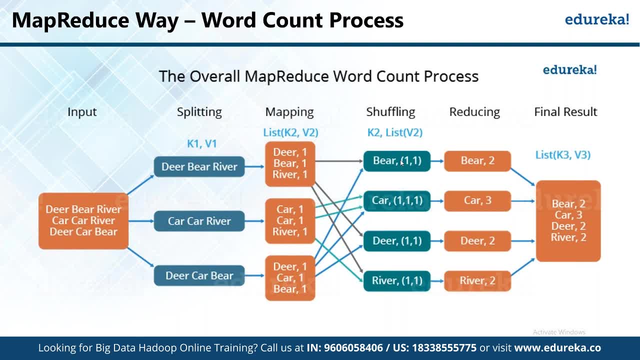 separately. and now, let's start now. We are going to reduce it. That means now we can calculate the total number of times these words have appeared. So bear has available for two times. That means it is to same of a car, It is for three, deer is for two and River is for two, available here. 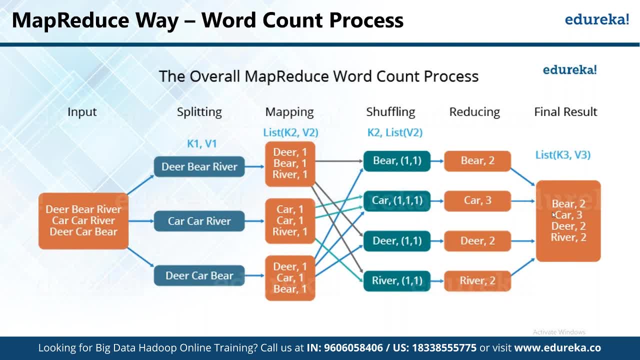 So here we can see the entire list being reducer and then we can get the final results as in: to bear three cars to do and to River, components available As a simple example of how the entire shuffling, how the entire entire piece of data set is splitted, is defined. 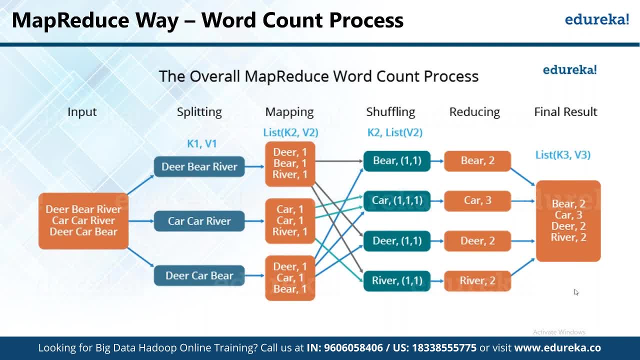 is mapped as shuffled and is reduced to get the final results out of the entire given data sets. Now, next, let's move further. So we have map review Now how we can use map reduce program using the young components of a Sephardi. now applications run natively in Hadoop. 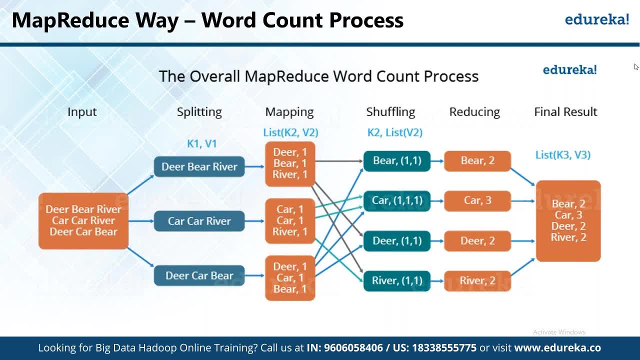 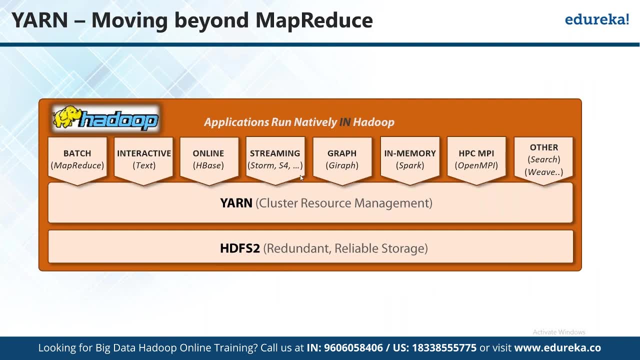 So, first of all, we have batch, So match is again done on top of my produce, and we have an interactive test for online. It is for edge base, for streaming. We use storm s4 for graph, for graph components, We use giraffe for in memory. 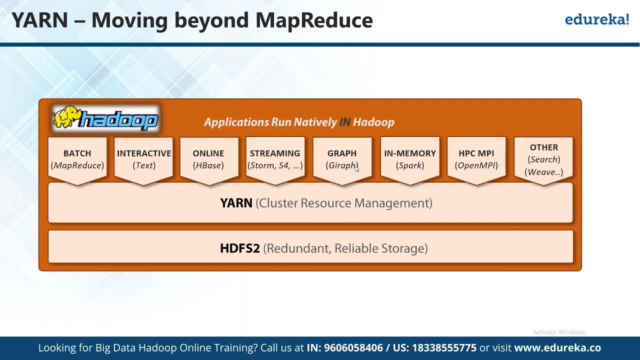 We use spark for HPC MPI, We use omen MPI and for all the others we use search. We went other components As a. as a company you can say they complete okay, and all these components are run on top of Yon as a cluster resource management. 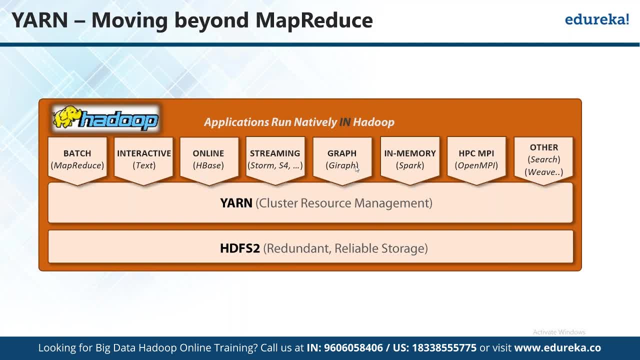 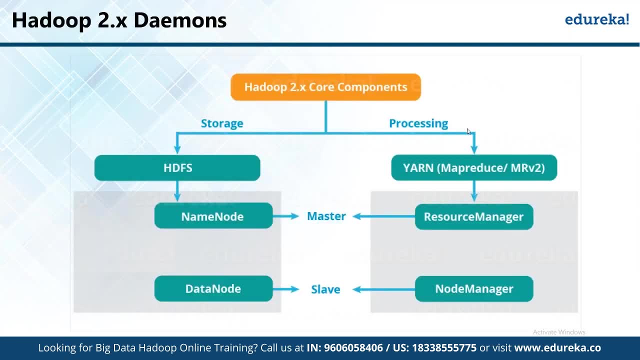 and then we have HDFS 2, which is more redundant and reliable storage Because, as you face, is barely used for the same parallel distribution of the entire data set. and Hadoop now, Hadoop earlier. There are two versions. We have Hadoop 2.0. 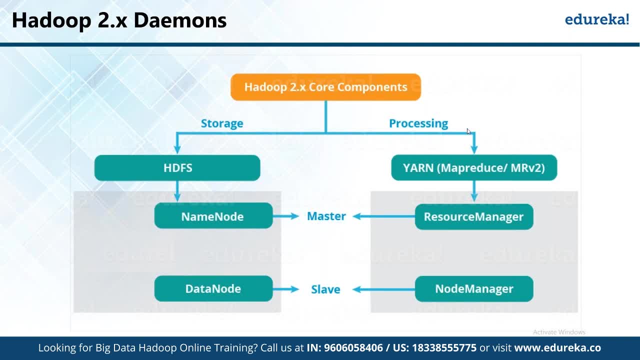 and then we have our previous version. Now in Hadoop 2.0, we have again for storage. We use the entire This component where sgfs has name load and data load in terms of the entire architecture. So when you say data node here with beans, for example, 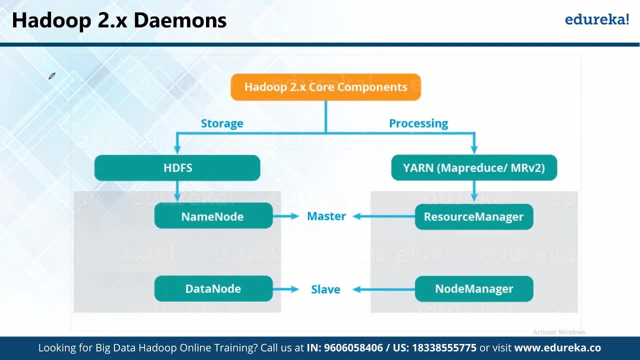 if we decide we had discussed the component of master and slave architecture. so Hadoop has a fall in master. We can create. we have master node has multiple data node. So we can say master node here is effort as name node. So name node contains a piece of. we can say at the entire metadata: 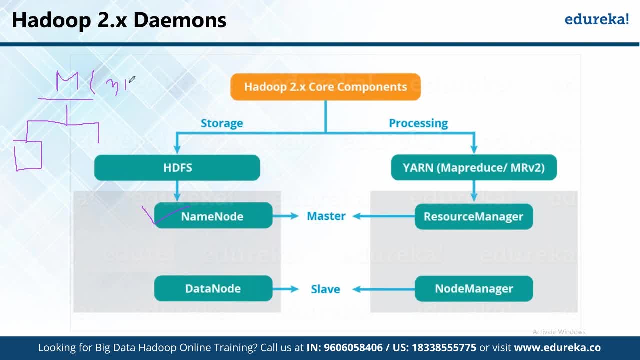 of how many master against how many slave nodes are present, How and what exactly are the locations where it is stored. That means this name mode is coming to act like a master node and each and every slave node, each and every slave node, For example, we are termed as data node here. 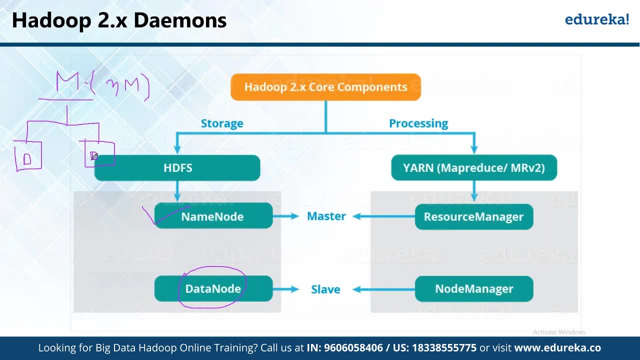 So the actual data is stored in these different slave nodes which are which perform the entire processing and be, and that's which, of individual data sets. and for processing part We use the yarn where we created the MapReduce program, and in here we have a resource management. 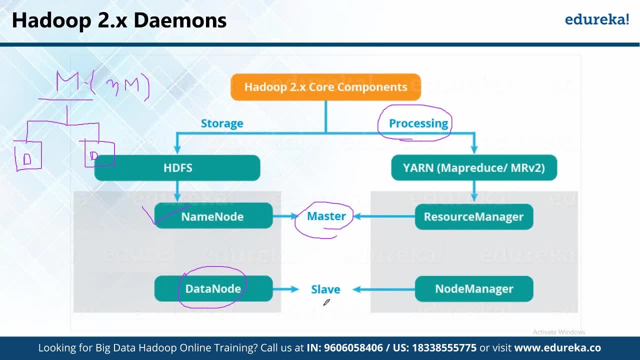 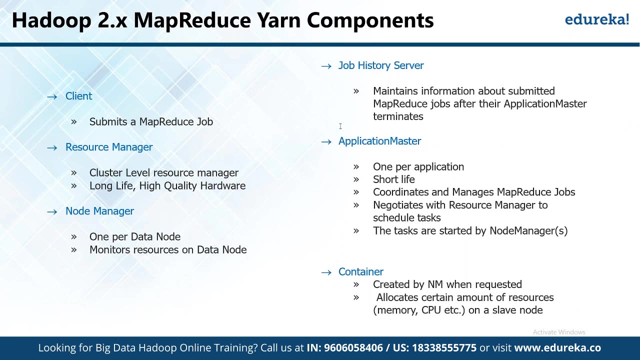 which is basically at like a same as master, whereas every node manager acts like a slave, even for processing. That's how we structure the entire Hadoop 2.0 component. Now, next component we have: now these are different components that even we are going to refer, so we can. so it's good. 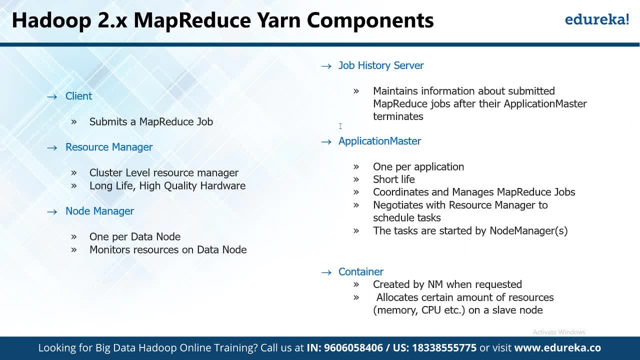 to have to simply divide, I can say to memorize the entire application used by these different components. So clients, now yarn has multiple components. first of all, clients. so client is basically used. who can say who's responsible for submitting a MapReduce job? Then we have resource management: minute resource manager. 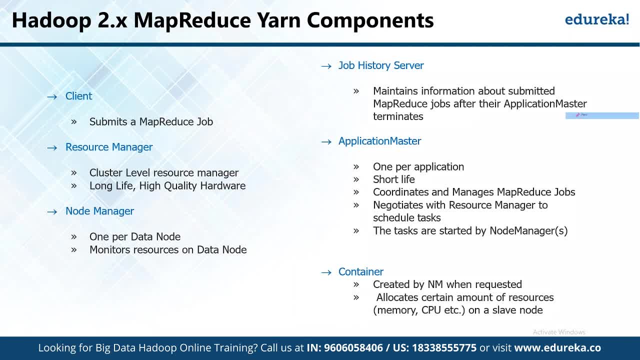 that we are going to refer as our M, So in and a further content, We are going to refer resource manager as our M, So our M does the cluster level resource management. It offers a long life and how to hide high-quality hardware, whereas then we are going to have node manager, node manager. 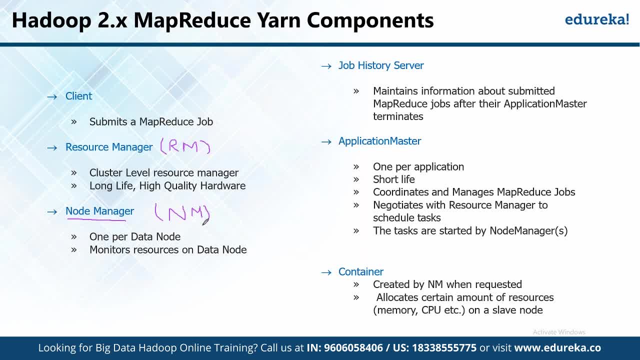 refers to nm. node manager refers to nm, where we are going to have one per data node. So for every data I know it is going to be attached to at least one name nodes. name node as in master node. correct, Because without master they cannot be any slave, correct. 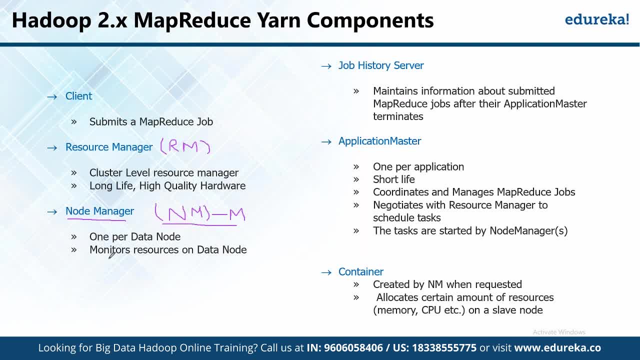 That's why we have to have at least one per data node available and which monitors the entire resource on the data node. That means how much data is present and how it is going to be processed one by one. Then we have job history server. 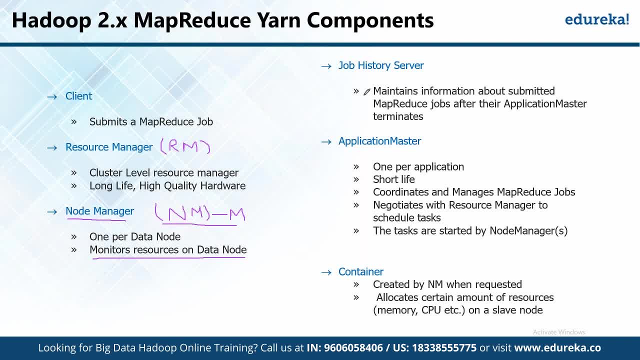 So it maintains the information about a submitted MapReduce jobs after the application master terminates. So I. so after the entire application master terminates, it is still going to retain the entire job details. Then we have application master that we are going to refer as AP. 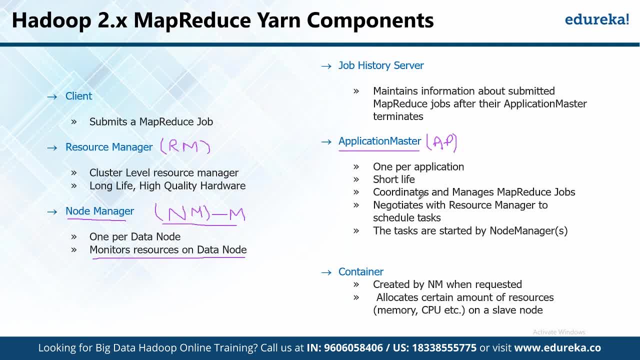 so application master again, they can be only one per application as a short-lived it. The main job of application master is to coordinate with and manage the MapReduce jobs and it simply negotiates with the resource manager, as in the Masters, to schedule the task. 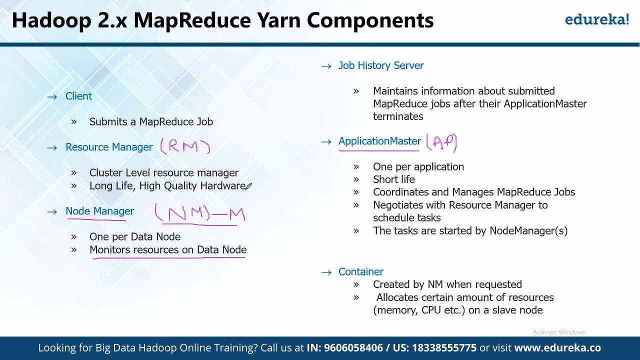 and the task are started by the node managers because they are the official data nodes, And then we have container. So again, these are created by the node managers when requested and they allocate certain amount of resources that we have: memory CPUs, the storage capacity for honor slave node. 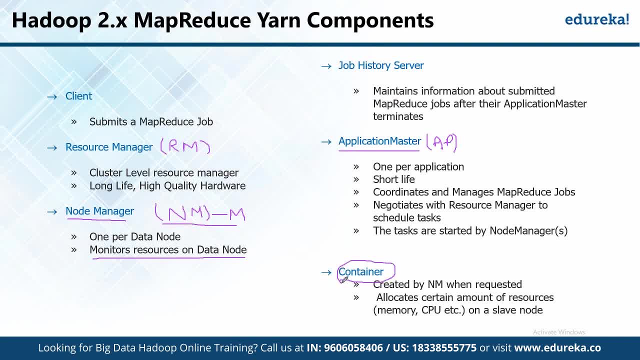 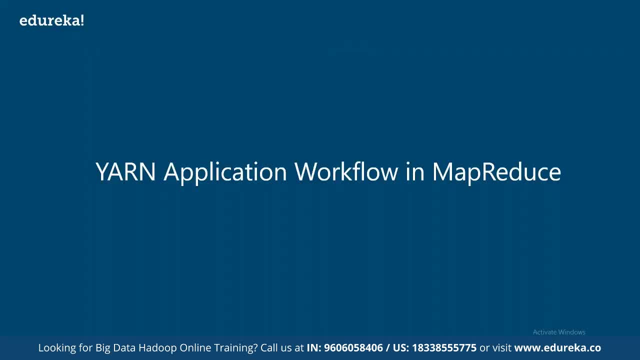 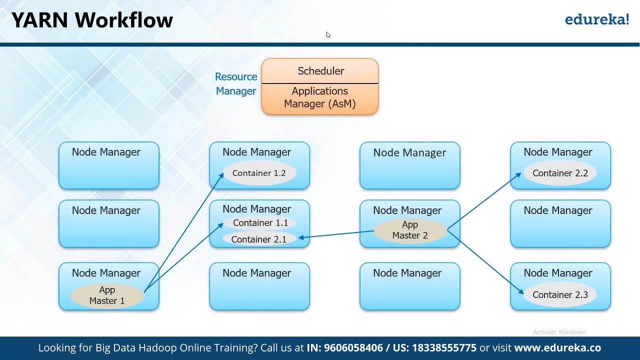 So they- basically they are responsible for the primary of these container base code that we can deploy on top of slave nodes, as in our data node available. Now let's understand the entire yarn application workflow in MapReduce. So, first of all, the resource manager again. 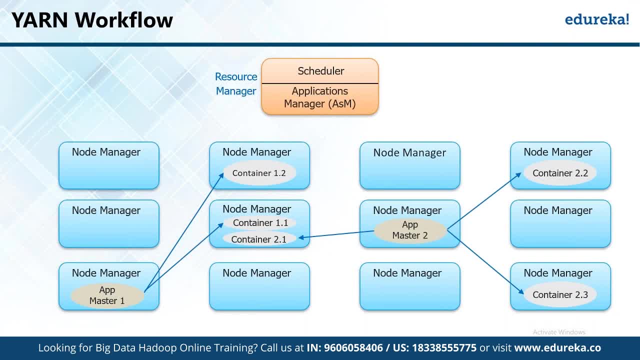 we have scheduler and then we have applications manager, called as ASN. For example, here we have a node manager where the application master is available. So it is going to create a container using the node manager and, again, node manager is going to decide on how many containers are going to be created. 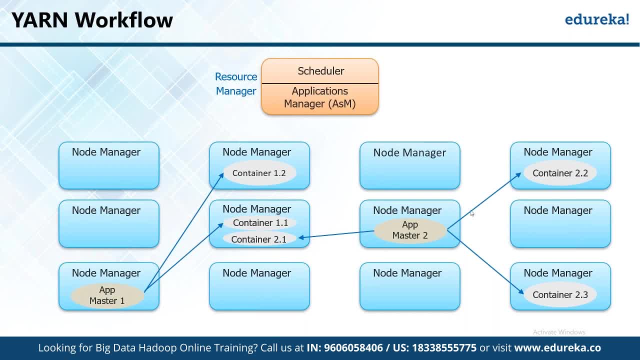 and then they can simply decide: I'm here in here. The node magic can also contain the entire master to, as in it can create multiple containers as you seek for deployment of, against the maintaining of the entire application code. here That means if we have to install this in a better terms. 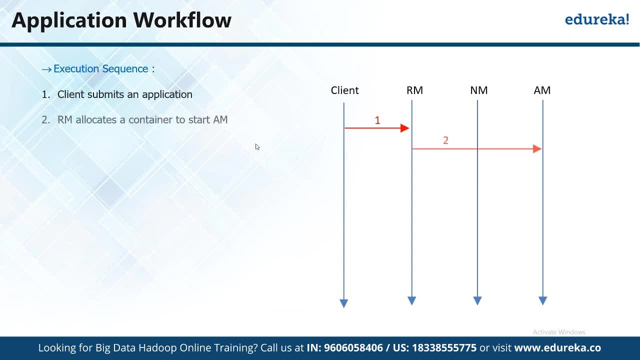 then, first of all, the client summits the application and then the resource manager allocates a container to start the application master. So am refers to the application master. So application master is going to be triggered by what? by the RM itself, and then application master simply gets registered. 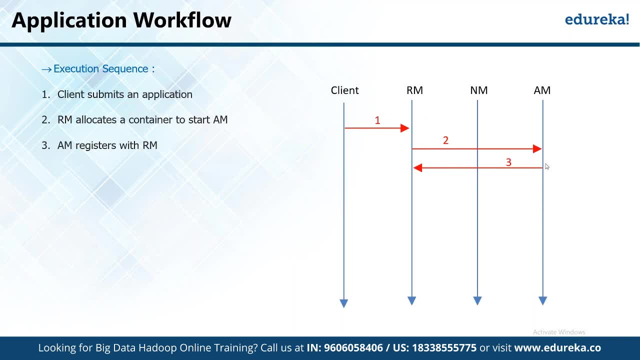 with the RM as in the resource manager. but the resource manager because once it is initiated it has to research cell to the resource manager. Then it asks not, and then it is going to ask for the containers from the given resource manager. So again, the request is going to be sent to resource measure. 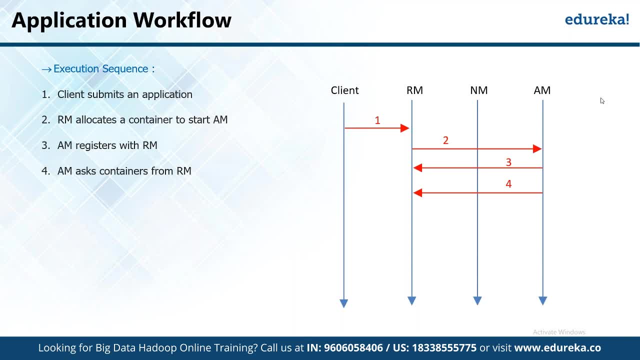 for the containers- availability- and then the source. we can say application map, measure it or it notifies the node managers to launch the containers after the request has been sent to the source manager, because the allocation is going to be done by the node manager itself, and then the application code is executed by the. is it executed? 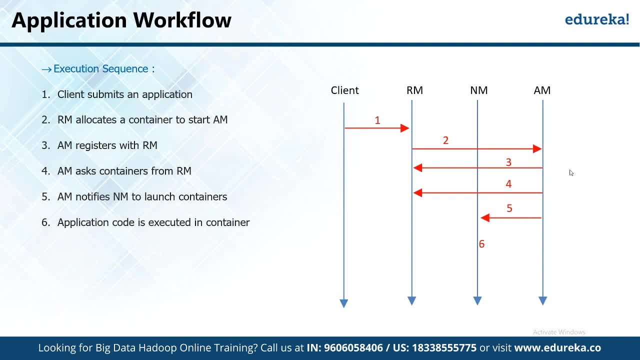 in the container And then only it gets passed on from and then the client recontacts RM and we can say RM or a or directly. You can also tell. we can say: contact the application master as well to get the entire application status update and then the entire state after the entire status update. 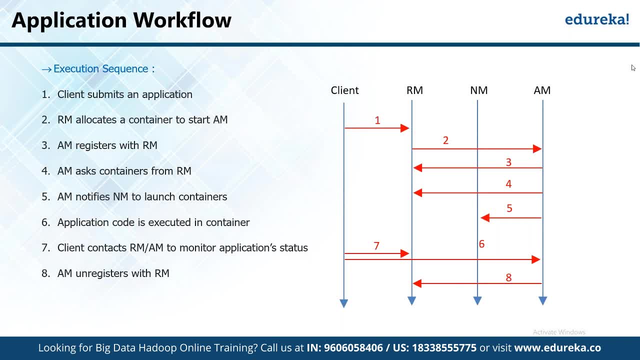 the application master is going to run register itself with the RM after the entire job is done. That's how the entire application workflow is structured in. Yeah, Now let's see how we can write the map or reduce a code one by one. 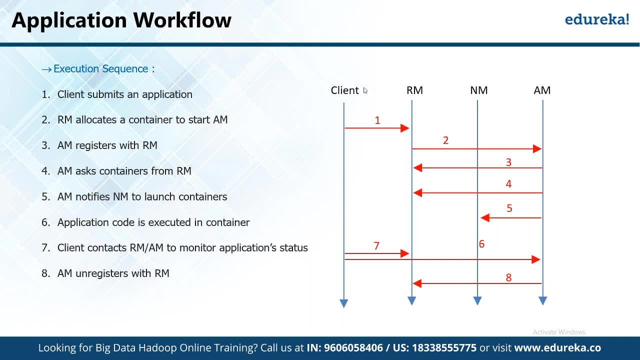 So we can use any of the code editors. so we can use any of the IDs to get started. So you can use any of the code editors or IDs to get started. So let's do that. Let's open up IntelliJ or Eclipse. We can use any of the IDs. 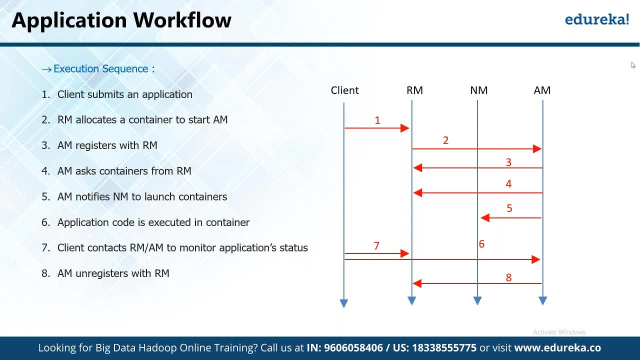 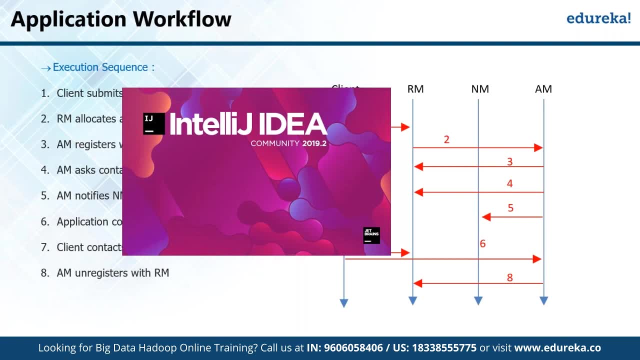 or we can also just get started in writing the entire map or reduce your code. Let this open up. So here we are. We're going to write separate mapper and separate, reduce a code one by one. Now this entire project has been configured. 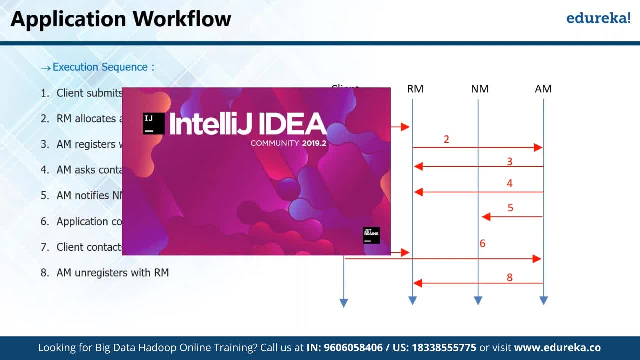 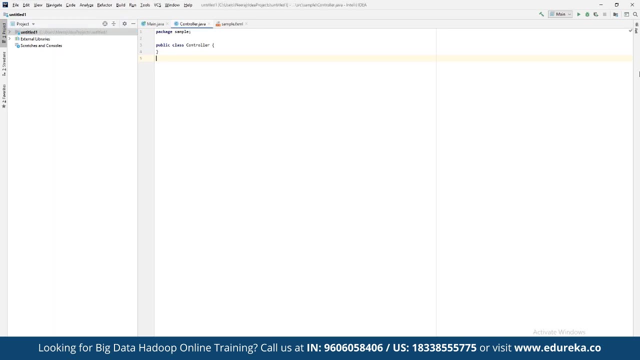 So you can start writing separate code for mapper and reducer both. So let's do that. Now, for writing the entire map and reduce a code, We can first of all import all the libraries that we have. The entire project is now currently available. not to give you complete sample of how we can define, 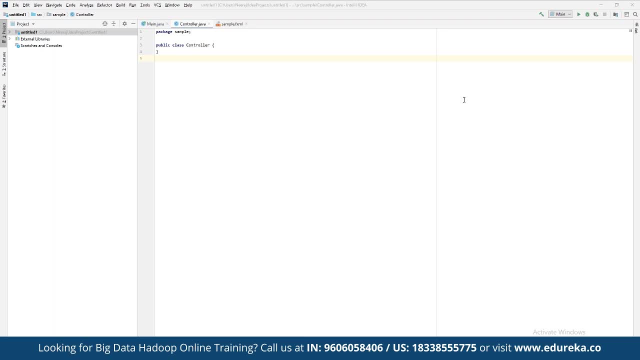 the entire mapper row, for example. Now the entire map reduce program has is divided into three different components. We have mapper reducer and then we have driver code. First of all, we are going to write the mapper code, Then we are. then we have to reduce it by using the reducer code. 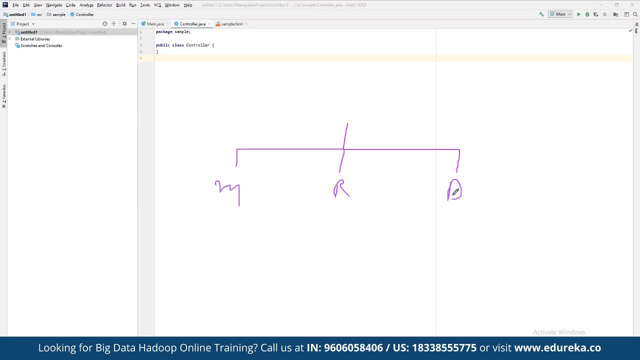 and then we have the driver codes. These three are core components for any map reduce programs. So, first of all, when we define- I'm now when we define- the mapper code. So let me give you a small example of how the mapper code is structured. 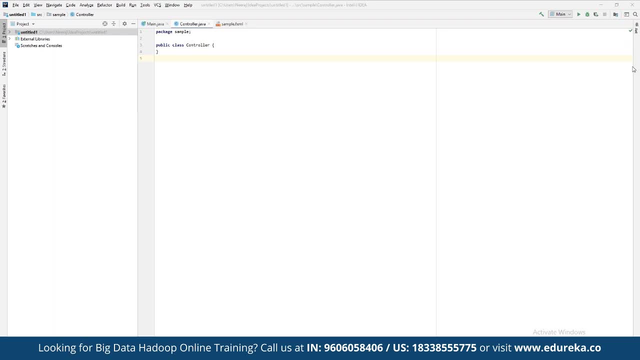 Now let's define the entire package first. So first of all, here we can define public static class map, For example. here we want to simply extend the entire properties for mapper that we are going to discuss, and here we can use a property for extends as a part of hierarchy. 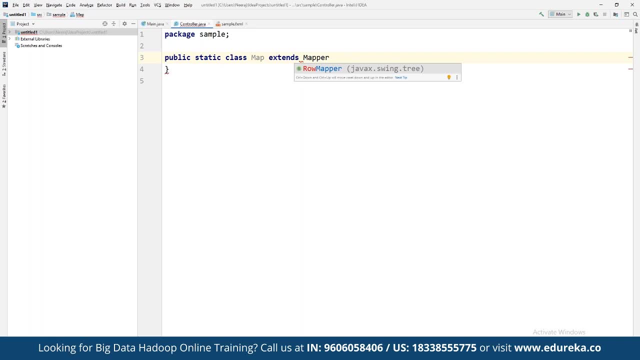 and then we can use it. Then we can extend this to the mapper code that we have. and again, here we can, if not for mapper, we can define long right table and then we can Define this for text. It is going to be in a text format. 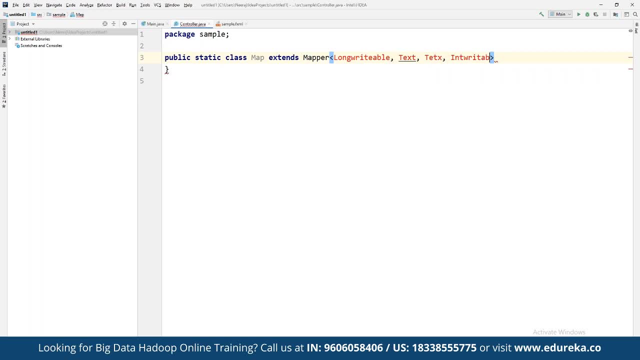 and then it is going to be inviteable. So here we get it to do to find the entire format in which its entire code is going to be. It is going to be text, not you know thing around. So here we have inviteable and then we can start to find the entire program. pointers. 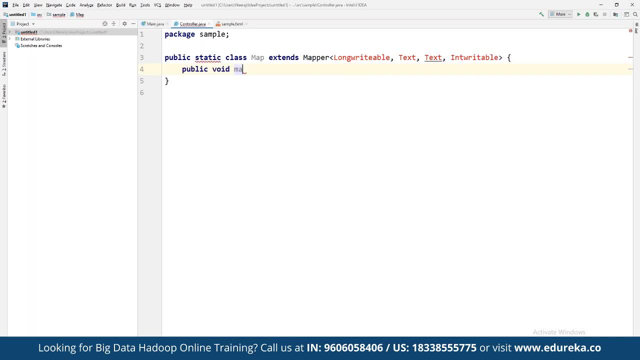 as public. Void me out here. We define, not map. you Let's start with the map itself and then we can define our. here We can define the property for it. So again, this is going to be long writeable, So you can long writeable. 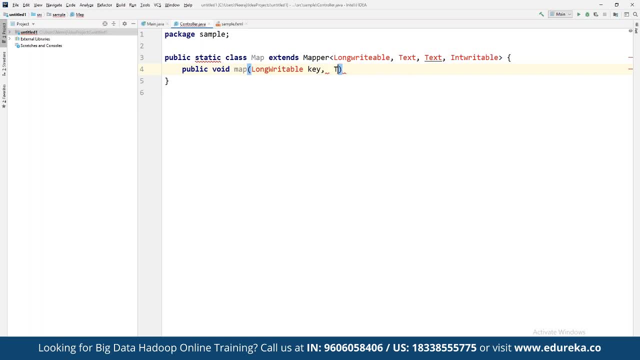 It is going to have a key, not long writeable key, Then it is going to have text value, Then the context and the contest again, if you have defined, and then we can. if I it throws the IO exception and interrupted exception. We give us a bit of space here. 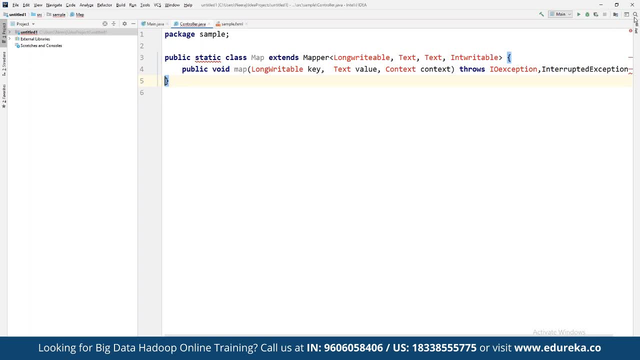 As interrupted, as interrupted exception. and now we can start defining the string line. or here we can down the exercise: We can define the string line, the string line where we can define the value, value for value to string, And then we can define string tokenizer. 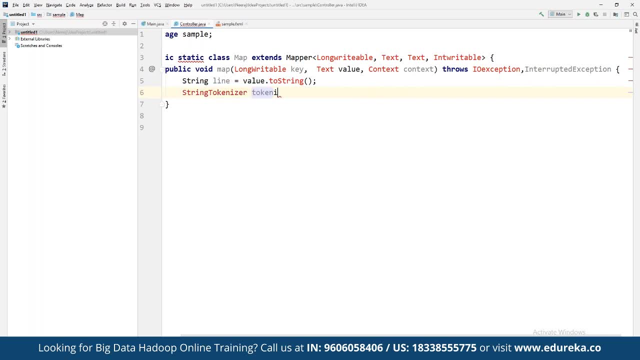 We can define string tokenizer, Stokenizer itself, Where we can create a new object as As new string tokenizer, your spring tokenizer for the line attribute. Then we can define while tokenizer. while tokenizer has more tokens, So here we can define a property for has more tokens. 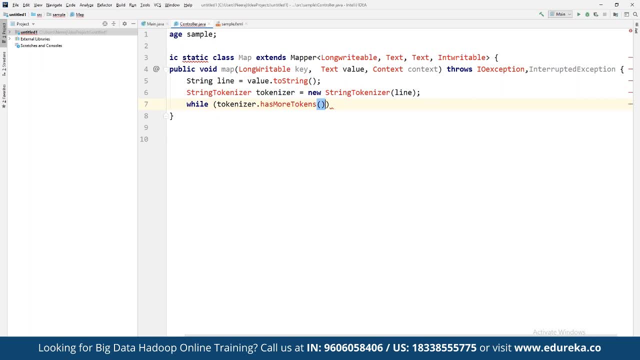 As more tokens, Then we can define. if it has more tokens, Then we can set the value value dot set For tokenizer. here We are setting the value for tokenizer, For tokenizer or next token. Then we can define the value here and then at the end we can define the can now here. 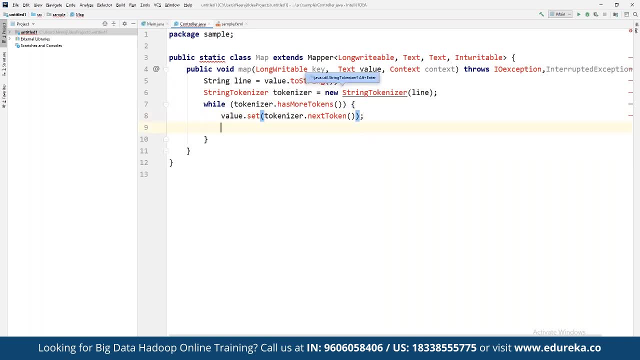 we can edit the and we can write the context value. So for writing the contest value we can find context, Context or to write We can find a value As new And write table, And here we can define index value as one. 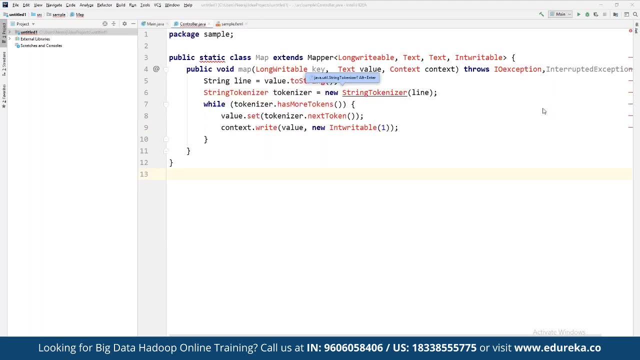 Now what we had: an we did a class, a class map that had that extends the entire class mapper, which is already defined in the MapReduce framework. And then we define the data types of the input And output key value pair after the class decoration. 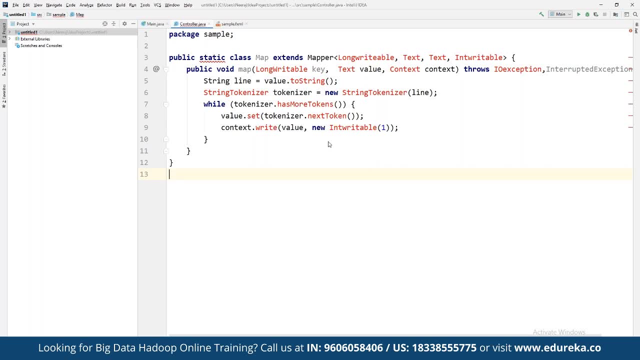 using the uncle brackets, and then both the input and output of mapper is a key value pair that we define and input We define. a key is nothing less but the offset of each and every line, like we have the long writeable and the value in each in individual line again, 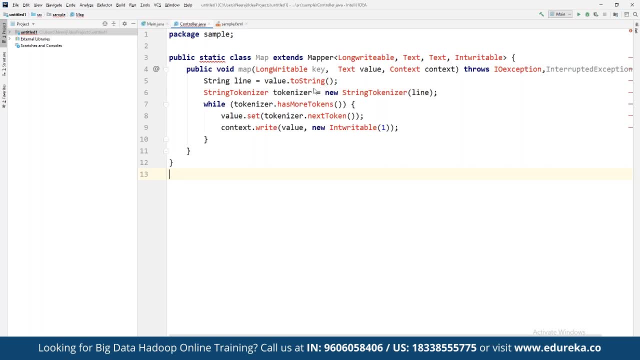 that is the component of text, and for output are the key is the tokenized word, And here we have hard-coded value in a case which is one, Let me declare as in writable. For example, we had discussed the component for dear for bear. 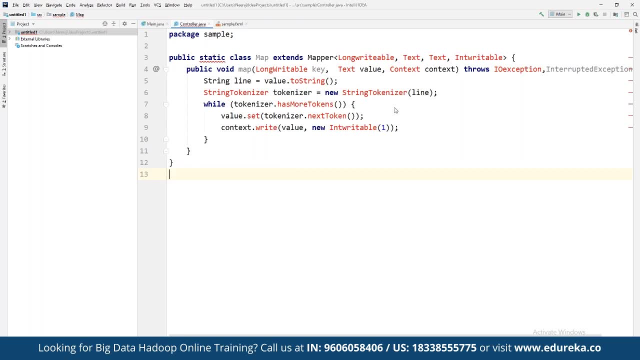 and as a value of one. and here we have written a Java code where we can have tokenized each word and assign them in hard-coded value equal to one as a part of the entire map of code. Now we have to write a reducer code where we are going to create a class reduce. 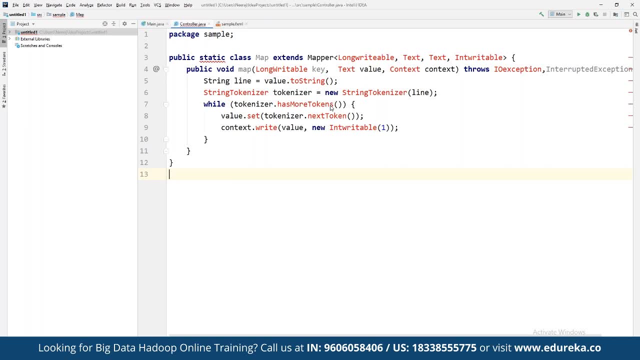 which is going to extend a class reducer, like that of a mapper, so we can write a simple or we can say reduce a code as well. So before we can now here, we can define the entire. for example, here, let's say, we are creating a class for word count. 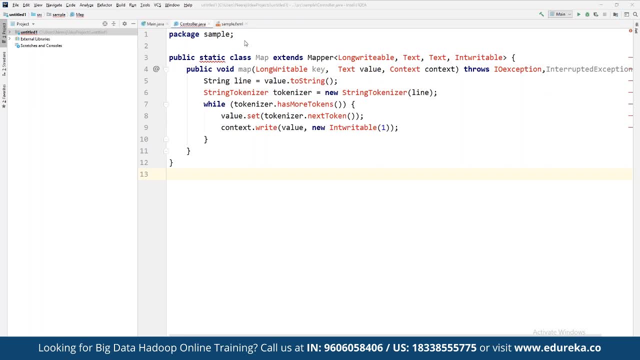 Let's do that First of all. let's, instead of doing the separately, Let's, import all the packages here, only so that we can get started. So here we can. they create a package for a safe for a director. Dot Map reduce. dot map reduce. 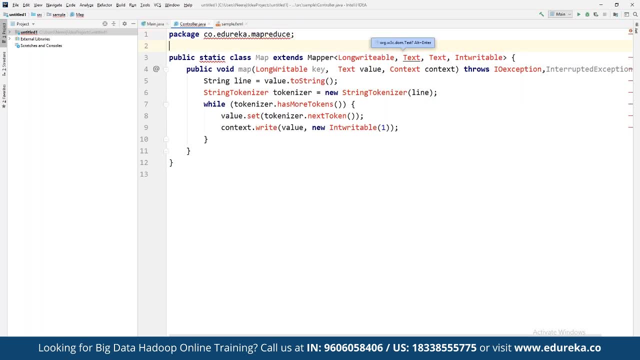 Now, here we are going to import, here We're going to import Java, dot IO, dot IO, exception. Okay, just to our conclusion: Let's support, Let's import all the components here at once, And it already very defined entire libraries here. 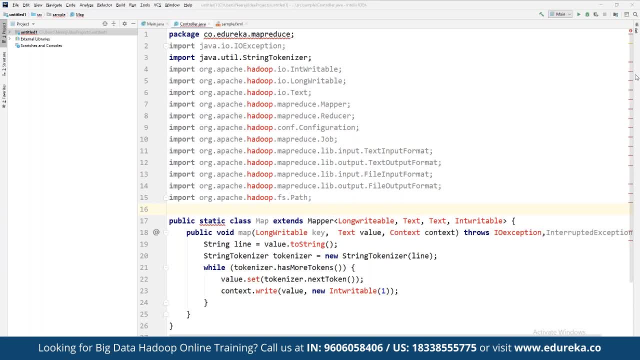 For example, out here We are going to create a complete class for, let's say, for word count. Let's say for word count, so we can do that. So are you able to see the screen syringe, as we've imported all the libraries here. 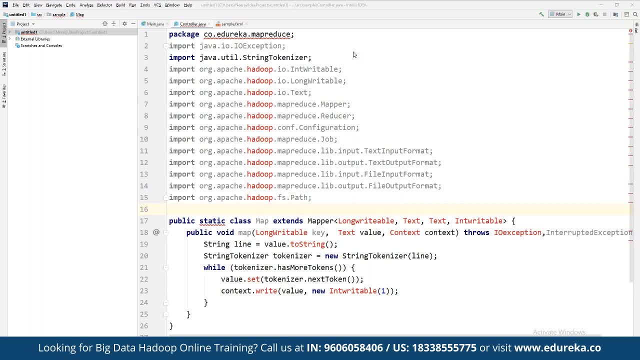 and let's do that one thing: Let's define one public class here for our public class for word count, a simple program that we are going to execute here as a part of the work or as a part of the word count. We can define the entire word count here. 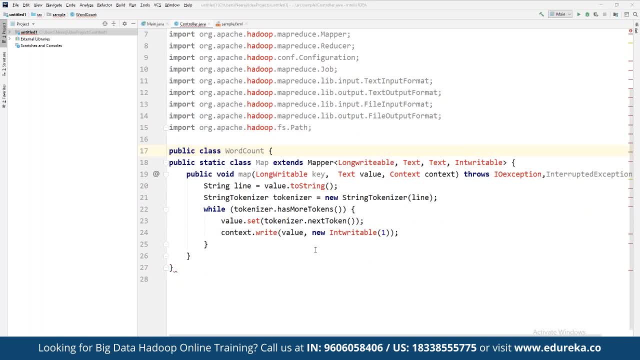 and for word count, and Sylvia defined the each and every public static class that we have structured your one by one. now let's do one thing on here: We can define these, reduce a code as well. So for reduce a code, We can define. 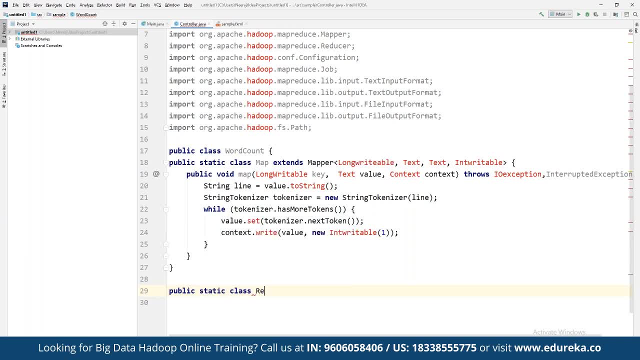 Another class, public static class- we can define is, as by the name of reduce, where we are going to extend this reduce from reducer that we had to find a reducer and from it is going to be: and writeable and as a format of, in the format of text. 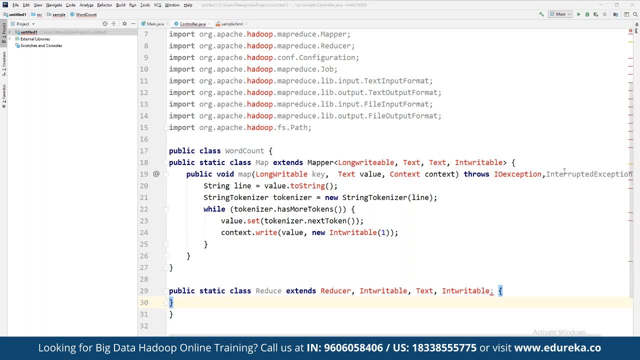 I'll give you already declared in variable again. All right, Now, once we are done, we can define the component for reducer that we are going to create here. So here we can define public void reduce. that's the finest as public void reduce, where we can define the text key. 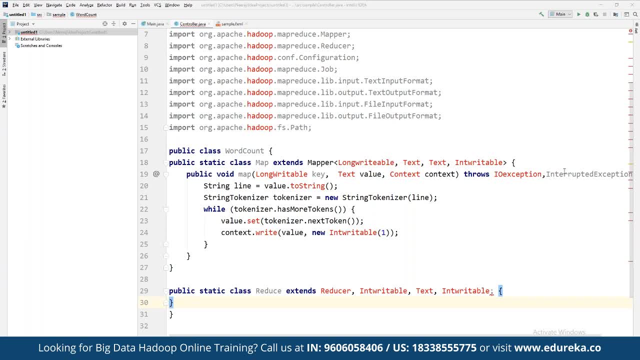 I get is going to be a table again, It is going to be in writable, and here we are going to define the same values context as we define in the previous example. All right, So now, once you define that here we can define: throws I exception. 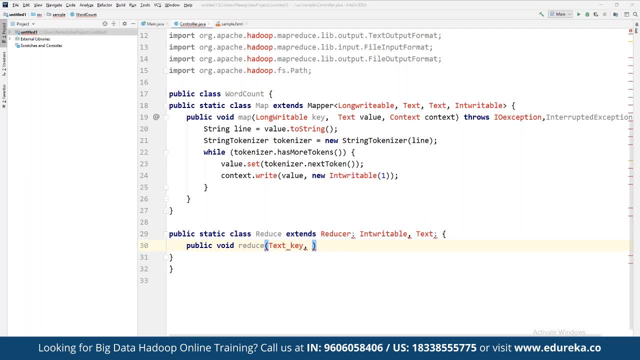 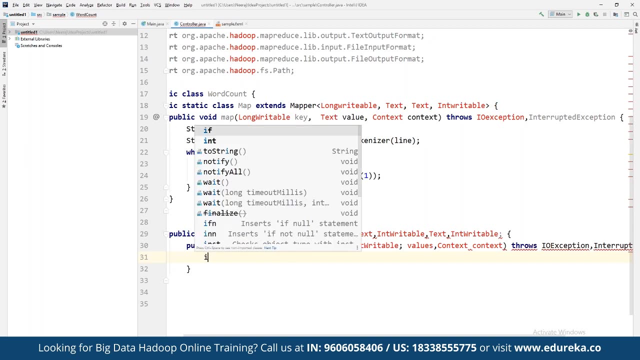 As in traffic section, one by one and after into the exception. here we can now, here we can define the component for the same reducer that we are going to create. So here, initially, we can define the initial value to be zero. So, since we are going to create for our word count here 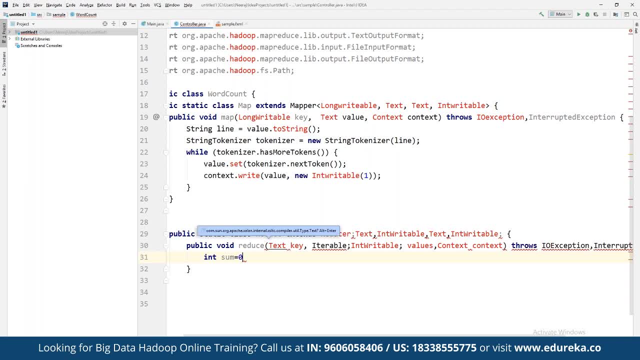 we can, we can define, and some should be equal to zero, and for in writable and writable X, where we are going to store multiple values. So for in writable X values we are going to go for, some should be, because here we are going to find the entire word counts. 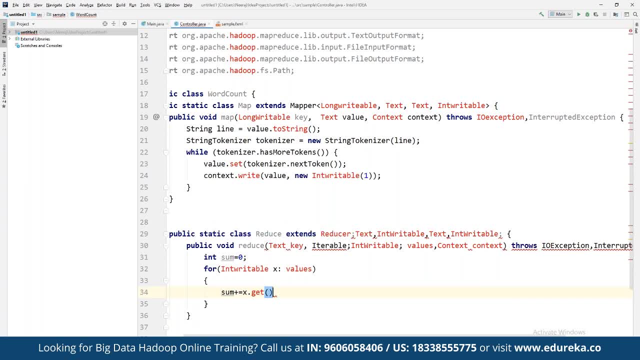 We have the sum should be X, which we are going to use the get code for, and then we can define the context. and then we can define context, then we can define the right for the given context, not for texture, for right, where we can find a key, value, key when them the end. 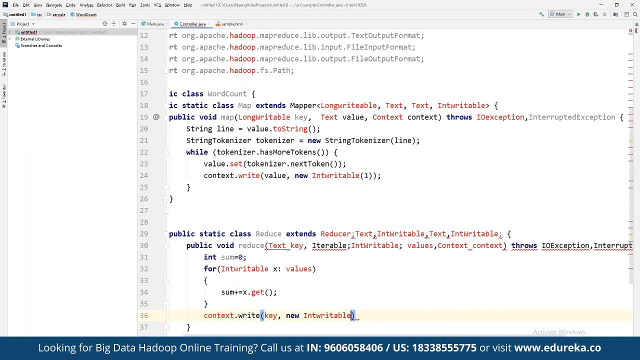 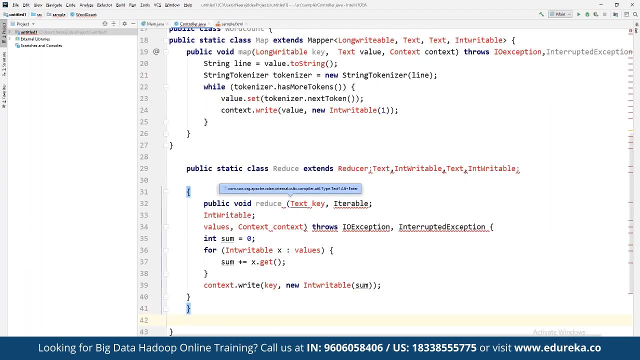 then here we can create a new And writeable very in this value is going to be some, or the incredible is going to be some here Now. next is we are going to Define the in case you want not. next is we can simply Define: after mapper and you so. 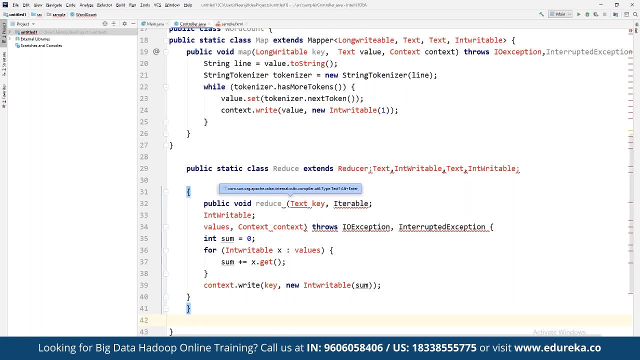 then we can Define the entire driver, the entire driver code. So for driver code we can Define the entire configuration. We can Define the entire job class. For example, here we can Define public static void Main and here we can Define string. I guess where we are going to declare. 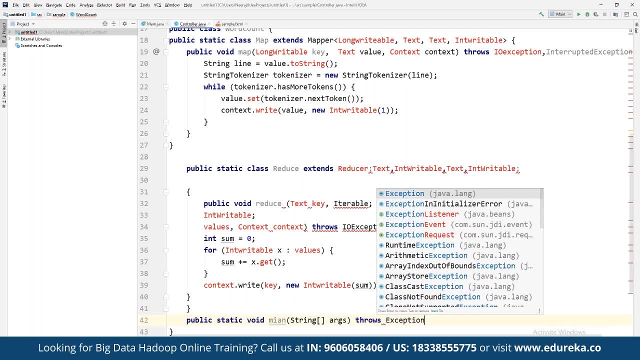 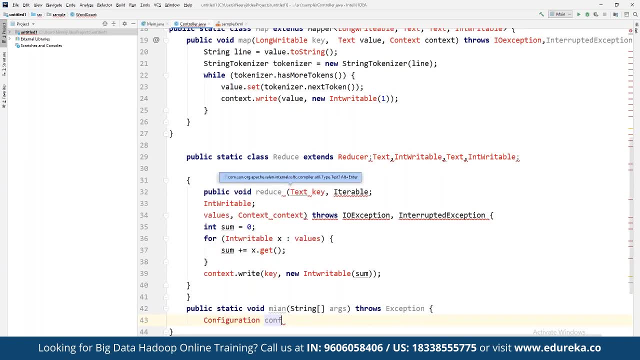 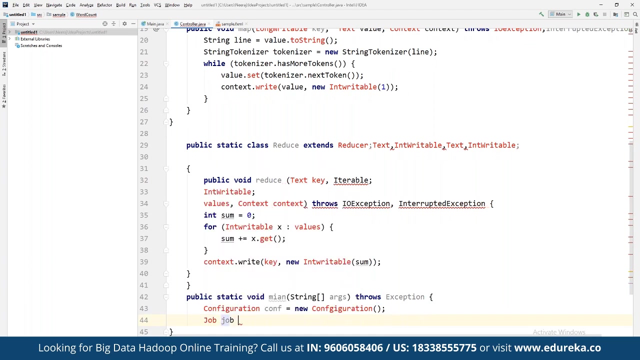 it should throws an exception where we can provide configuration configuration. We're in this configuration. We are going to declare a configuration where new configuration And then we are going to declare a complete job. So here we can create a new job where we can configure. 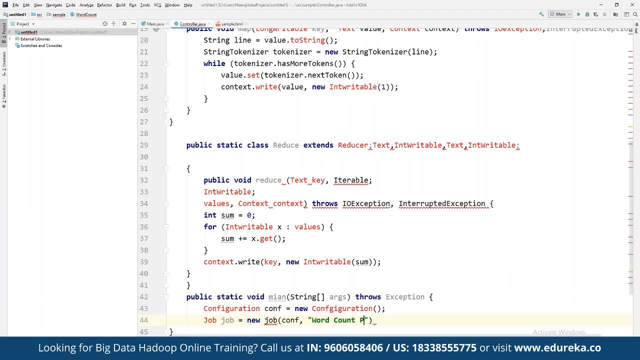 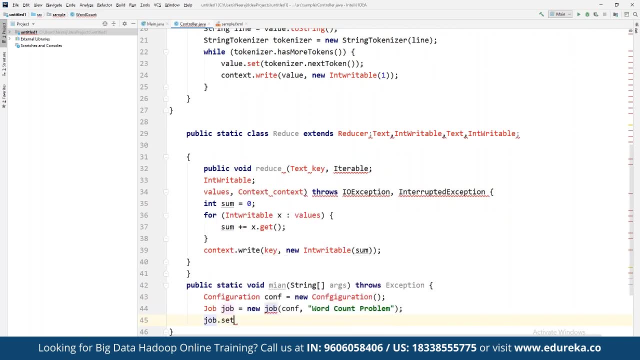 as suppose as word count problem, word count problem, And then we can, from the job that we have, we can use set jar here now. So here we can Define said Jaya by a class, and then we are going to use the word account, Word account or class. 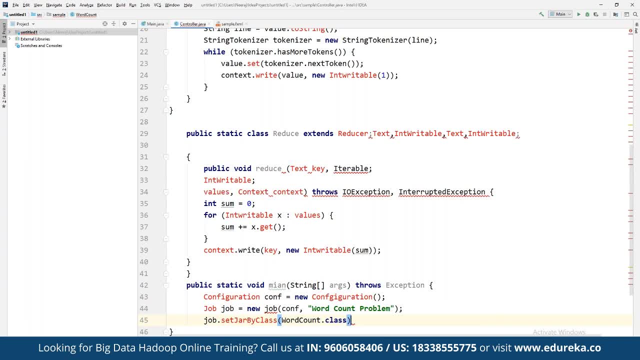 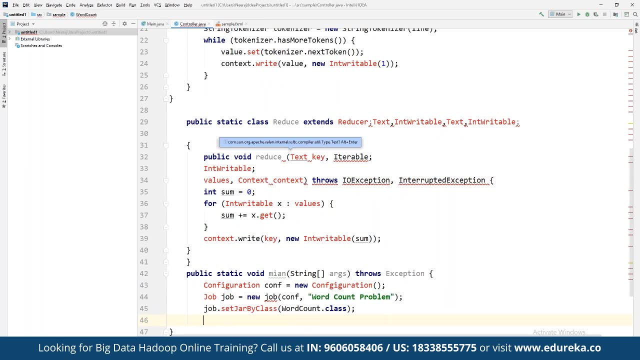 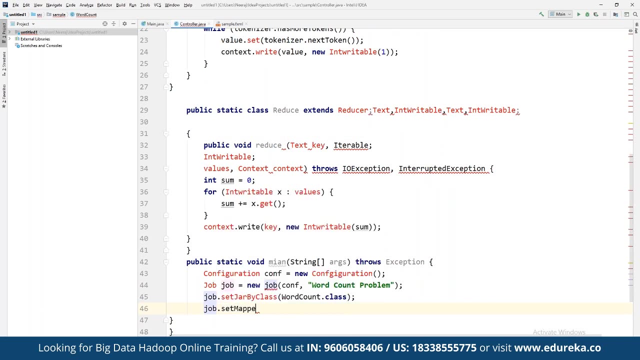 What condor class here? and then we are going to Define mapper, We are going to Define reducer, We are going to Define the output key class. the value class would not one. so for support we can Define the map class here. So here we can Define job, not set mapper, mapper class. 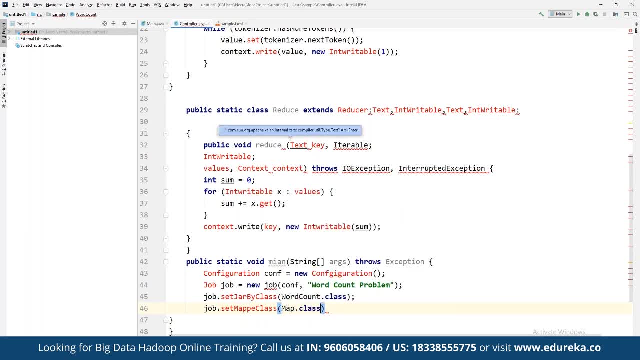 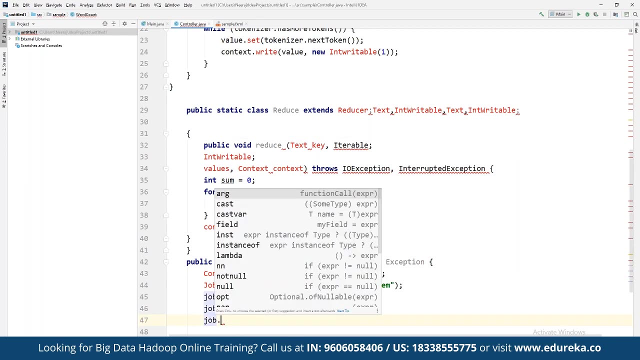 So mapper class is going to be map dot class And then. so here we are set mapper class. I think we missed on. them are yes. So here we have set mapper class, So it is going to matter class. next We are going to do to set up the reducer class as well. 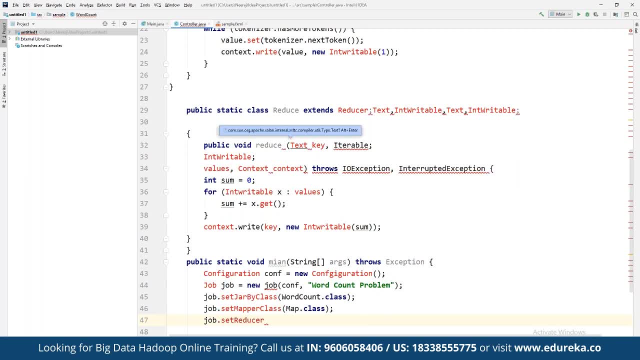 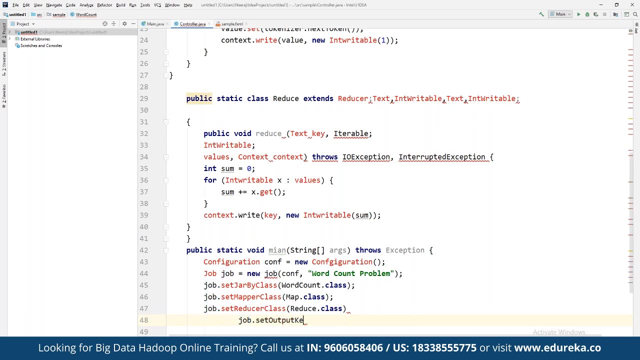 So set reducer: set reducer class where we are going to Define reduce dot class. You're going to use a use class, then we are going to create the output key class. So here we can use set output key class Where we can Define text, the class for text. 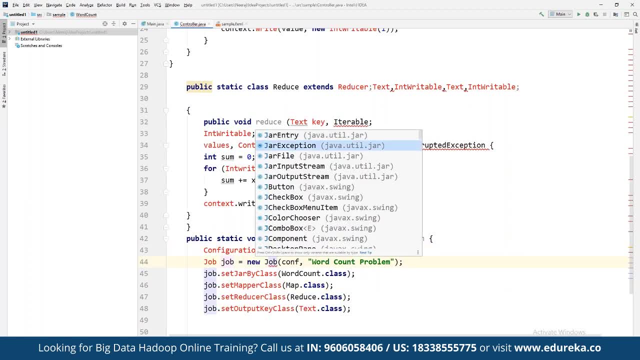 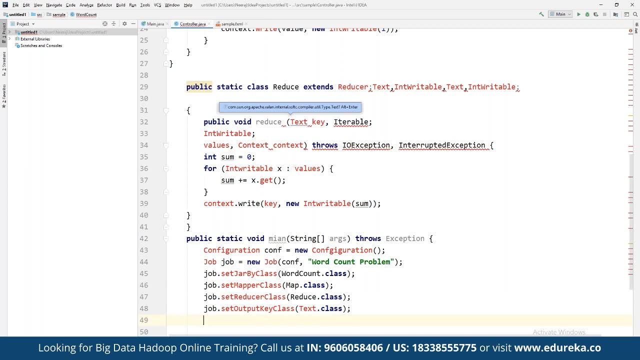 Let's keep it to uppercase, as we have used lowercase here. And then we are going to declare the output value for class, The set, the output value set, the input value and the output format as well. So here we can Define job dot set, output value class. 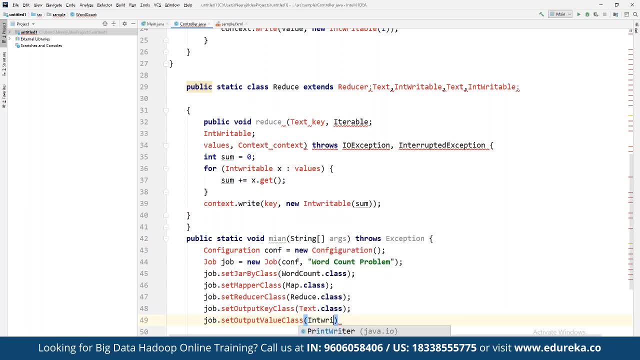 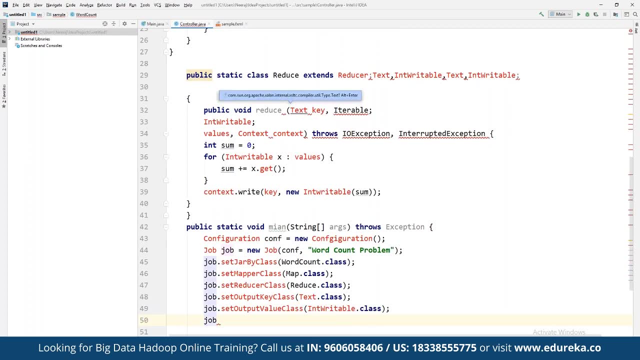 Here we are going to Define the same in variable class itself That we have used earlier in variable dot class, and then we are going to use job for the input format. So here we can use job dot set Input format class where we are going to declare text input. 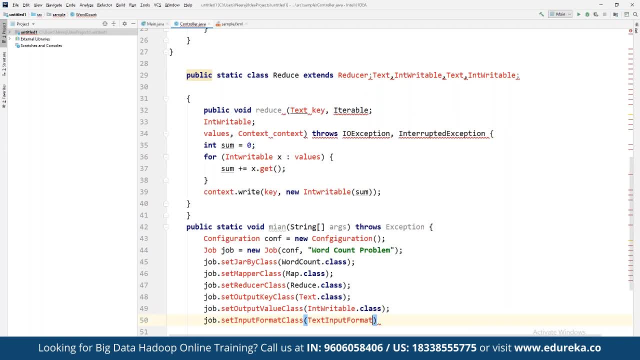 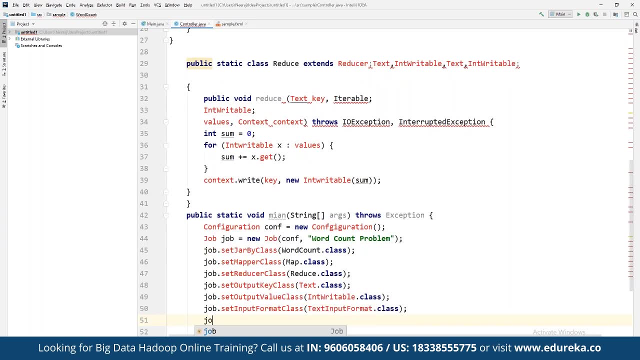 Text input format class, And then at last we are going to Define the text output from our class. So here we can tell job Dot set Output Format class. We are going to clear text Output format- Thought class, And then we can Define the path here. 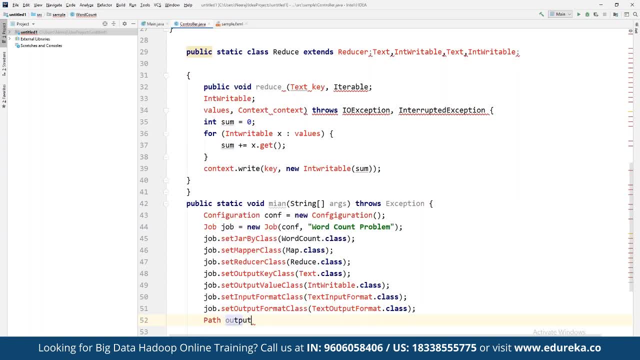 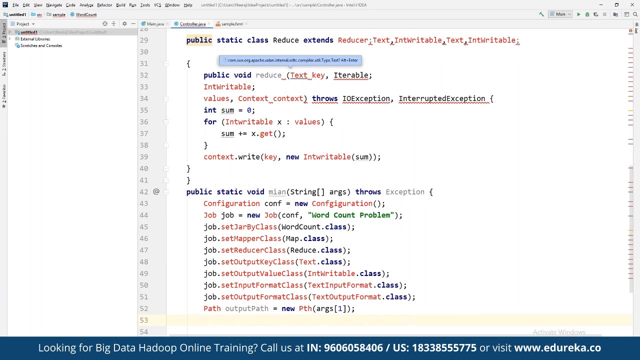 Here we can Define path. Part should be for output, But where we can create a new object here for part, I'm in the argument to find us one, And then here we can configure the path. Now, here we can configure the input order path. 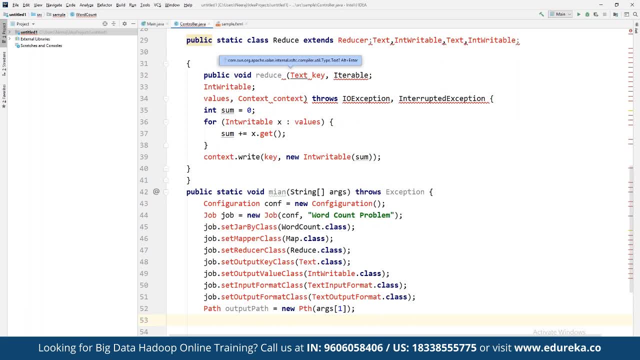 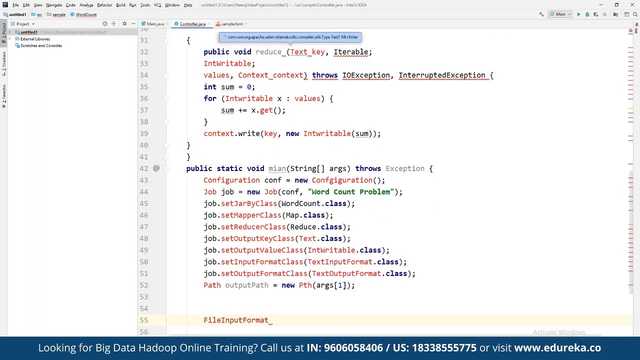 from the file system into the job. So for doing that we can Define file input format. So here we can Define file input format, Dot, and input Path. So basically, what we are doing is simply configuring the input output path from the file system into the job itself. 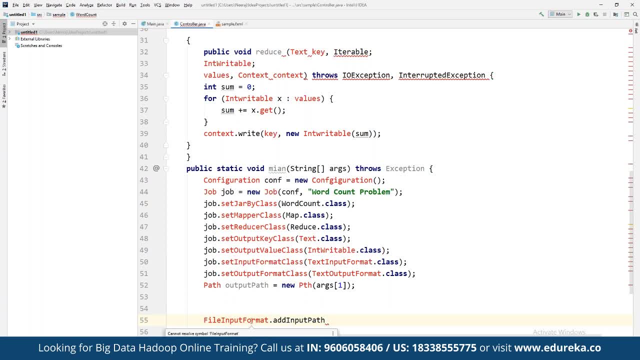 So here we can enter file, input path, file into format dot, add input part And then we have we can declare the job type- Here we can declare job And new part where we can declare the index value as zero. So here we can declare the index value as zero. 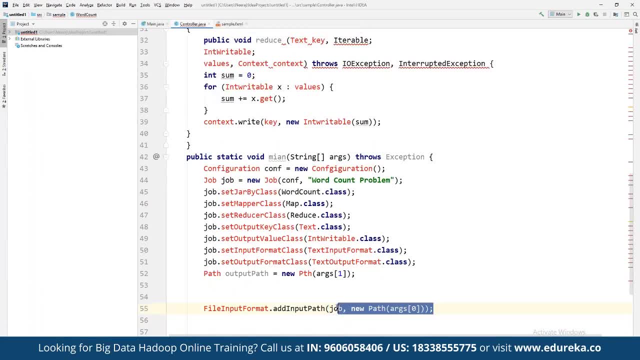 Same way we can Define for output path as well. So let's copy the entire parameter here. So here it is going to be for output, For output path, And here we can also create a new path. But here we can Define the index value to ask one, not as zero. 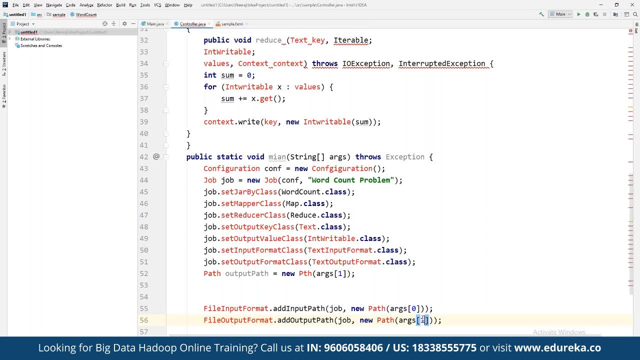 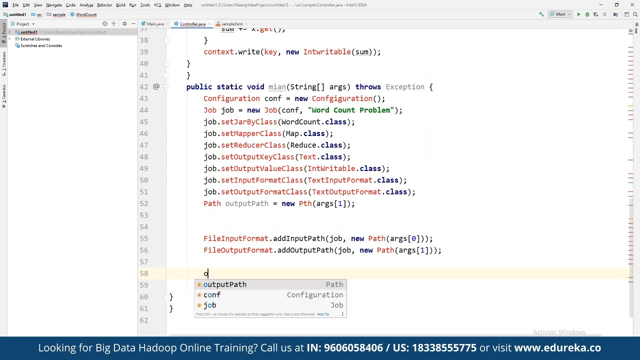 but here as one, and then we can delete the output path automatically from the HDFS, so that we don't have to delete it Explicitly. we can declare that particular path for us. So for doing that we can Define output path. So here we can Define output path. dot get file system. 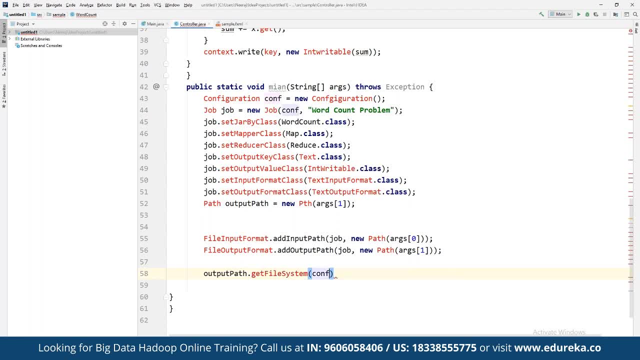 where we can configure it, where we can configure it For deletion. show: here We can use delete output path so that we don't have to delete it from the HDFS on our own, and then we can simply exit the job If the flag value becomes false. 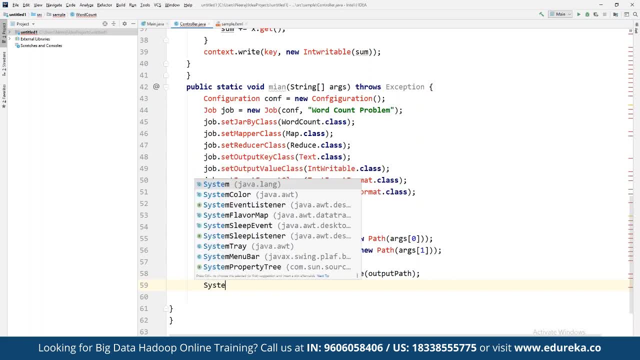 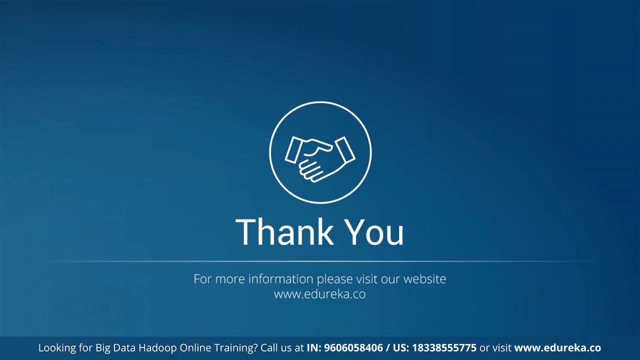 then we can exit the job. and for exiting we can use system dot exit, and here we can Define job dot wait for completion. If it is true and the value is true here, then here we can Define the exit path. So, as it's almost time now, guys,